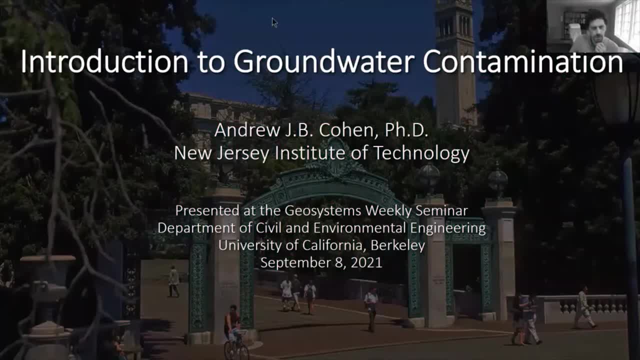 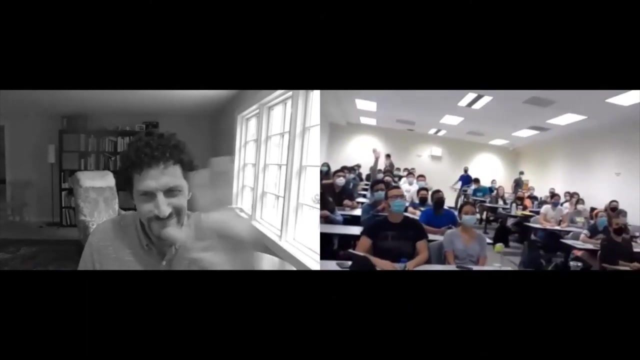 Okay, Welcome everyone. So welcome to our seminar. Let me turn my mic on. Okay. So, as I mentioned in my announcement today, our speaker is joining us via Zoom. I'll turn this around so you can see everyone that we have here. So we're here, Andrew, in the screen. So everyone is here, excited for your talk. 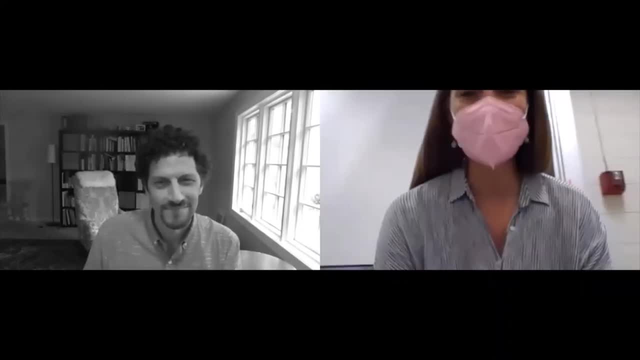 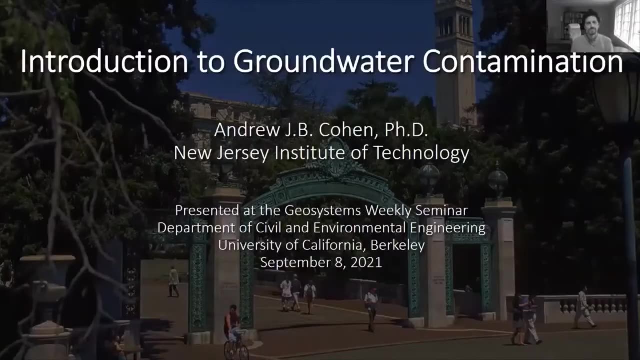 I can turn it back again for questions, But thank you so much for joining us And I think we can get started, because we had a little bit of a delay making sure that the sound was working, but it is working now, So I'll just leave you to it And then I'll just turn off the lights in the front so we can see the image really well. 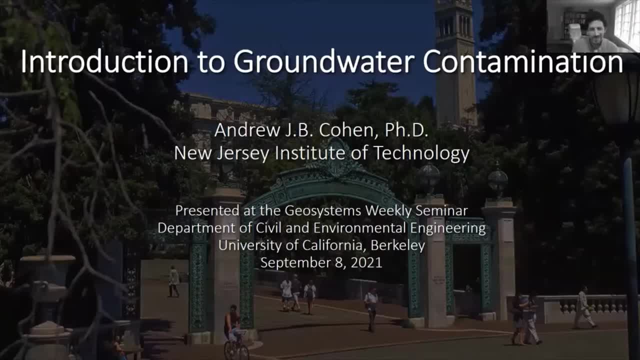 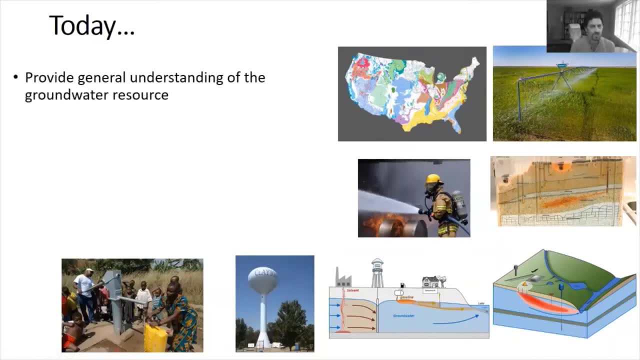 Go ahead. Okay, great Well, thanks so much for having me. It's really a pleasure. Today I'm going to provide a general understanding of the groundwater resource And I'm particularly going to focus on the presentation of visuals to present groundwater basics and also fundamentals of groundwater contamination. 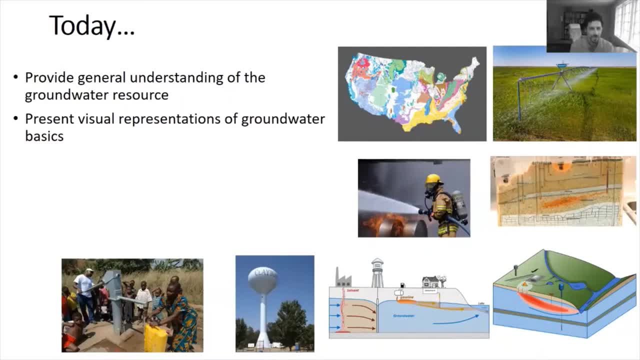 One of my assumptions here is that many people in the audience Are not very well versed in groundwater and groundwater contamination and, and I think so, covering some of the basics will be helpful. As part of this learning, I'm going to present short animations of various groundwater contamination scenarios. Many of these are based on real sites. I'm in the groundwater remediation industry, or environmental remediation industry, So I borrowed material from from sites that I've worked on over the years, over the past. 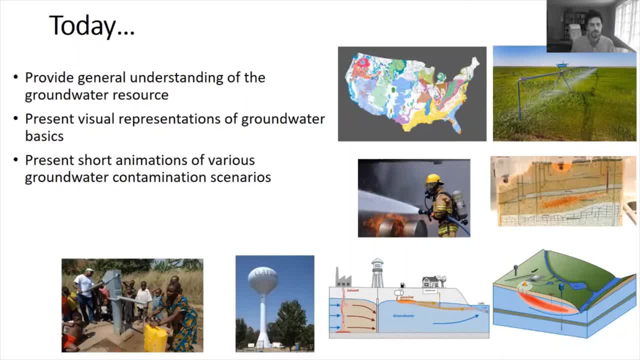 So I borrowed material from, from sites that I've worked on over the years, over the past. What is it? 2020, plus years, And I'm going to discuss the visualization and the context of conceptual site models, and conceptual site models are extremely important. 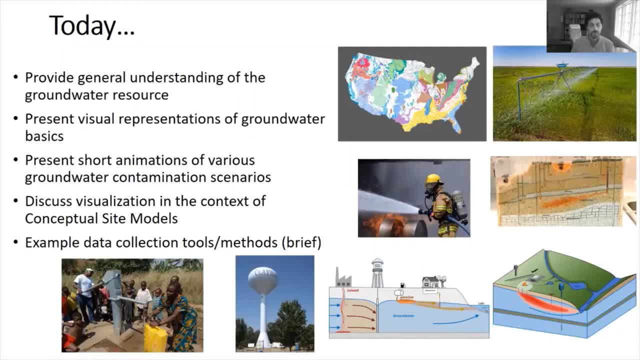 In the design of remedial systems or in terms of conveying environmental issues to stakeholders in general. and then at the end I'll just do a brief overview of what tools we use to collect the data that are being collected. I'll just do a brief overview of what tools we use to collect the data that are being collected. 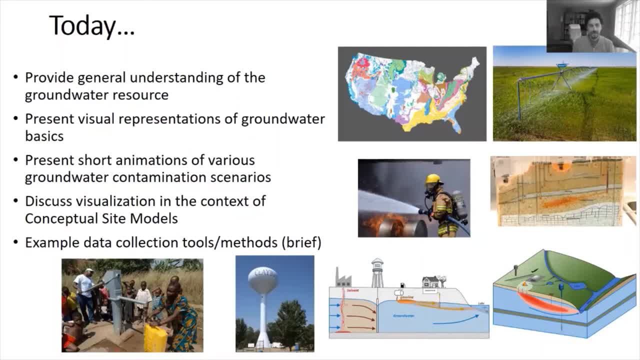 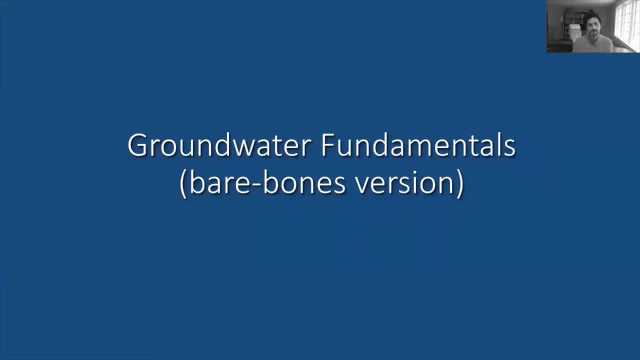 So I'll just do a brief overview of what tools we use to collect the data that are being collected, then used to basically develop these depictions and understanding of groundwater contamination. so let's go over the some groundwater fundamentals. this is bare bones, um, if you want. 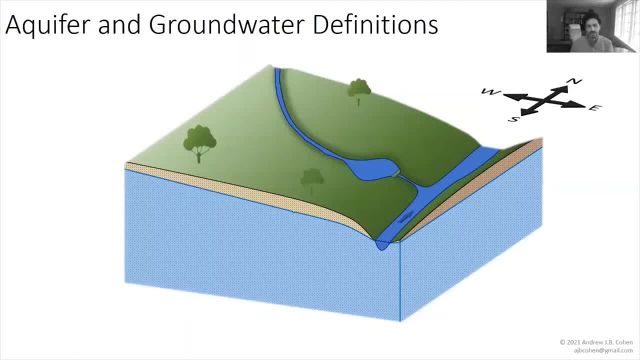 a deeper discussion. there's an online site with free material called groundwater or the groundwater project. that's gw-projectorg. i also have a book that's i co-authored on that, going over the basics of groundwater hydraulics, so that that could be helpful for you. 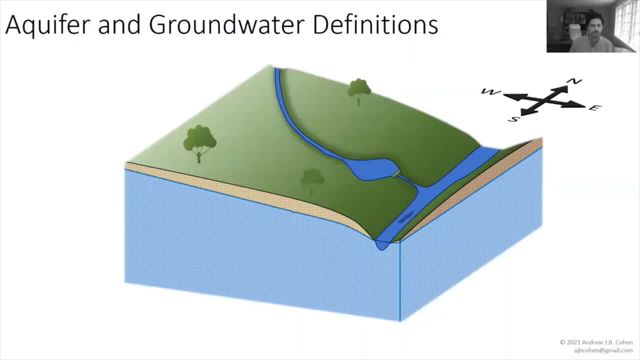 so just going over some some fundamentals here: aquifers and groundwater definitions. 3d oblique view of a groundwater system, also with the surface water body, reservoir and river, the voids in the soil of the rock beneath the surface, that part of the system that's filled. 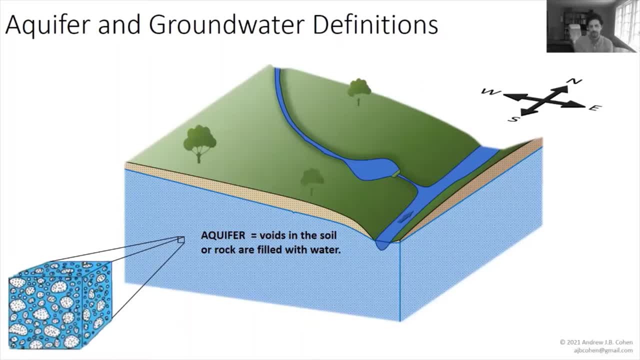 with water is defined as the aquifer, and on the left there i'm showing just a zoom in on the surface of the surface of the aquifer, and on the right there's a little bit of water that's saturated with water. so essentially we've got, in this case, let's call this a sandy aquifer. 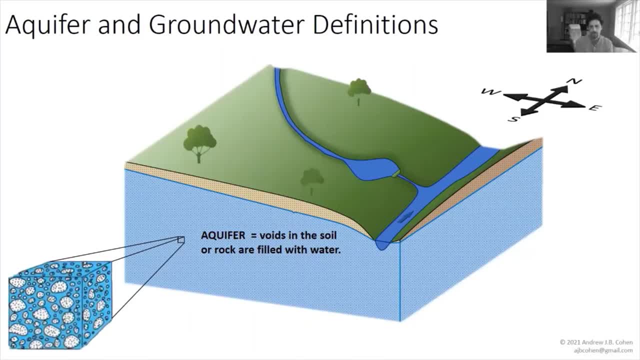 sand grains. in between those sand grains it's saturated with water. if that water is reasonably extractable, by wells for example, then we call it an aquifer and obviously water in this aquifer is called groundwater. that's our focus today. now i've i've mentioned that we're talking. 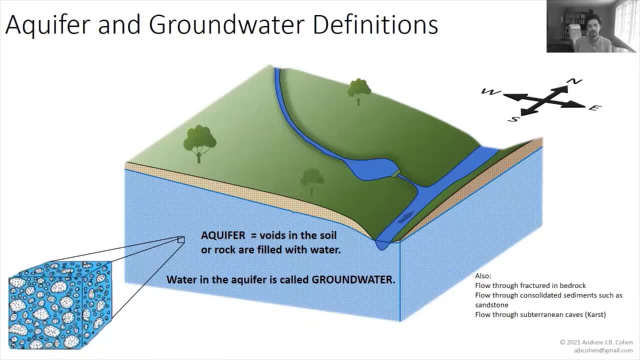 about a lot of around water, like sandstone, even a lot of other sediment, but in in all of the different areas that we could be actually talking about, you need to be talking about river water. that's an another important element of the work we're doing in the space. 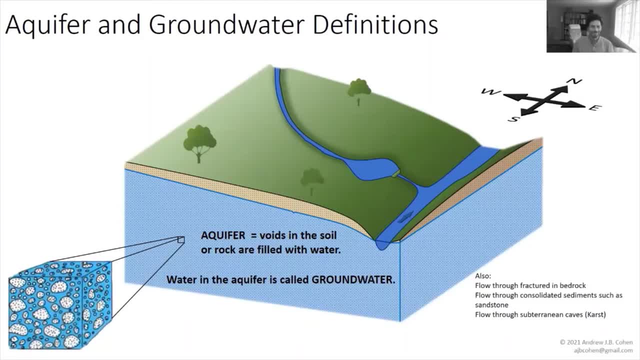 we need to talk about is the fall. the fall, and in fact this is really the first part of the project we're working on, and then the second part is we're looking at a second series of challenges that are facing us, so we're going to talk about this in the space and then we're 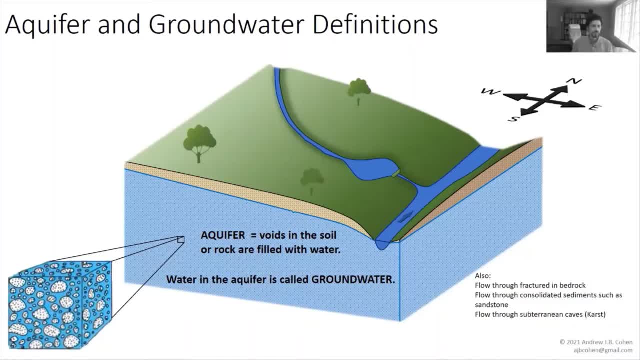 going to try to narrow it down and see if there's more resources people have that are going to talk about the next step. so this is about the one we had mentioned before. we talked about So that turbulent term comes off of all of our analytical expressions and the mathematics and the groundwater modeling. 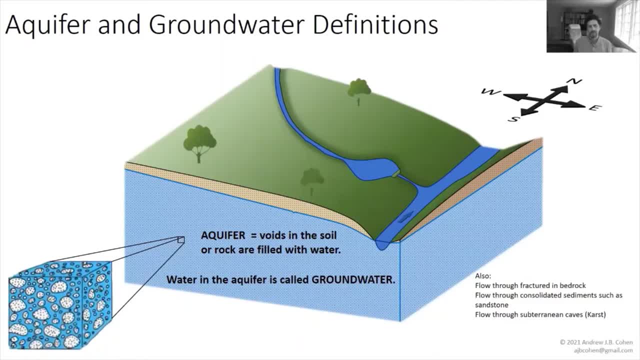 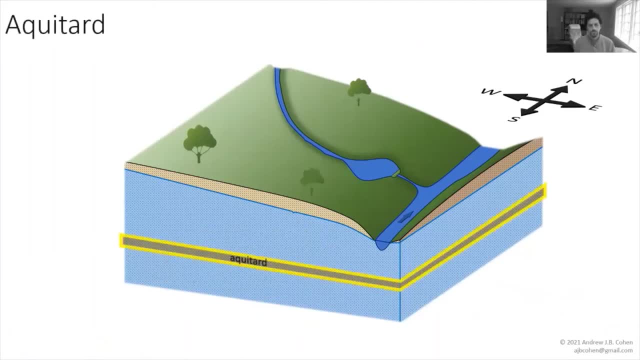 So when we talk about this, think about the contaminants migrating in the context of flow through porous media. Okay, now we can break up the aquifer, or the subsurface, into at least three different systems, right? One of them is: you have this aquifer and it's separated by a low permeability layer, which is referred to as an aquitard. 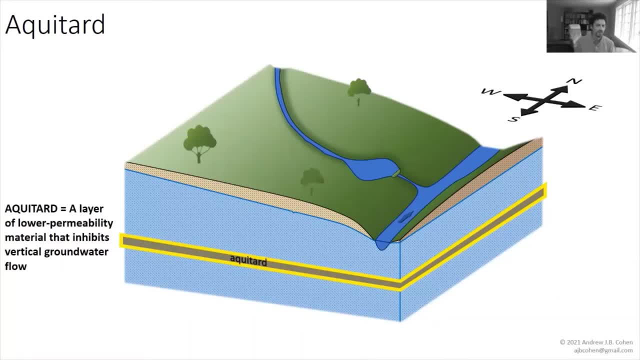 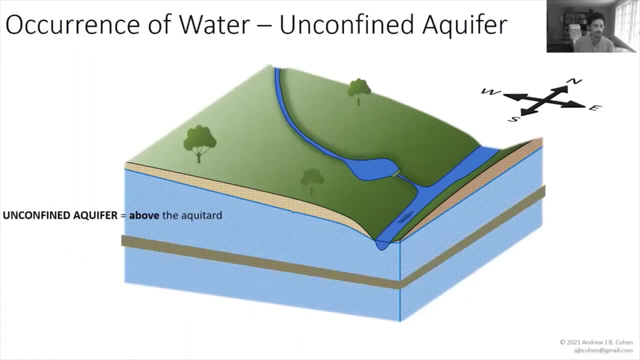 So that essentially separates or hydraulically separates these two water-bearing zones, or the parts of the aquifer And the portion of the aquifer above that confining unit, or that aquitard is called an unconfined aquifer. That saturated zone beneath the aquitard is called a confined aquifer. 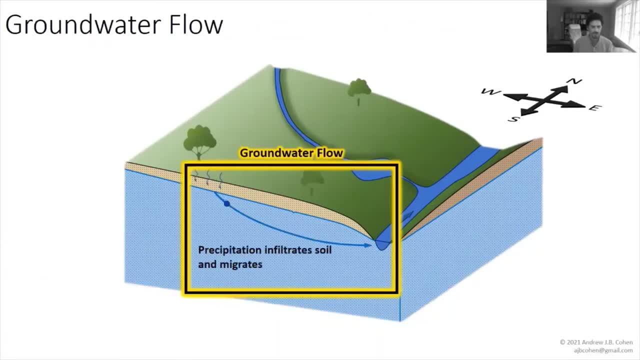 Okay, so here I'm just going over some basics. What's happening here? Where's the groundwater coming from? Well, it's coming from precipitation. Groundwater precipitates, it migrates downward and it flows towards surface water bodies which are at lower elevations in terms of water level elevations. 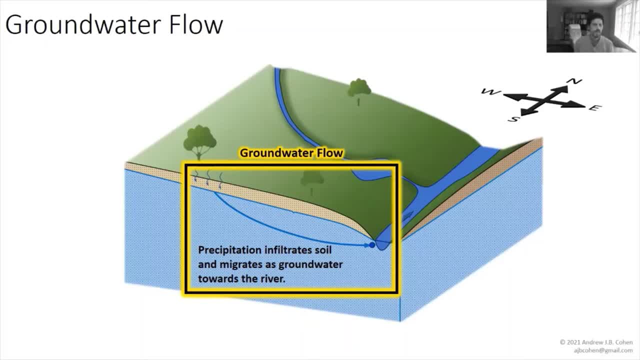 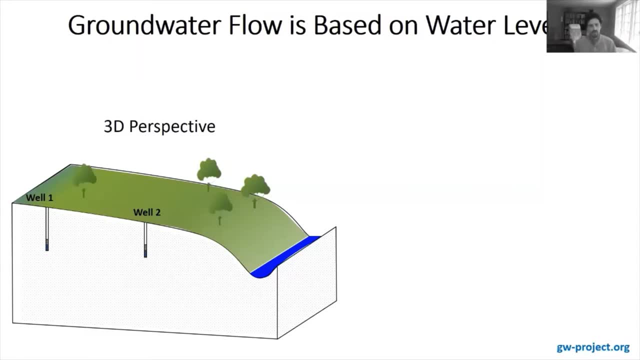 So here are just some of the fundamentals, some visuals And groundwater flow. what's groundwater flow? Well, we've got Darcy's Law, we've got hydraulics, but basically we're talking about saturated flow here. Take a look at this 3D perspective chunk of land here. 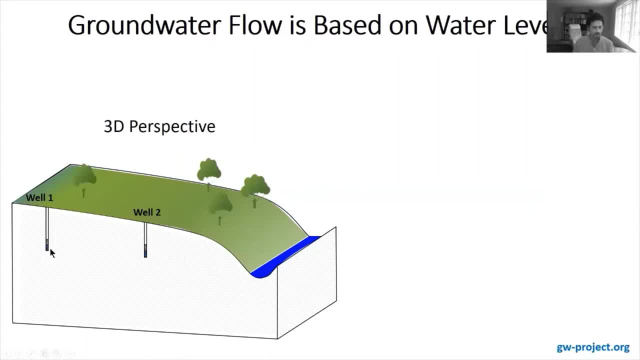 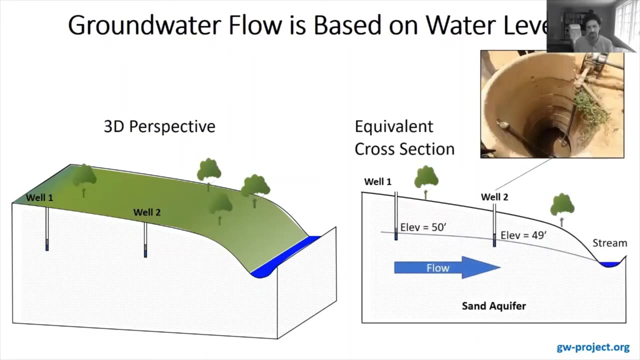 We've installed some wells. In the wells we encounter some water. at the bottom, in the screened interval That is, there's a slotted pipe, essentially through which water can enter. Typically, when we depict groundwater soil contamination scenarios, we'll use a cross-section. 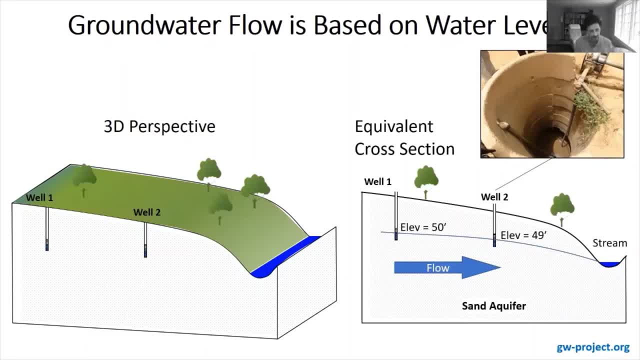 So what I'm showing on the right here is kind of the equivalent cross-section. I just kind of rotated that and this is kind of the schematic where we typically look at. So again I've got the two wells and the water levels. 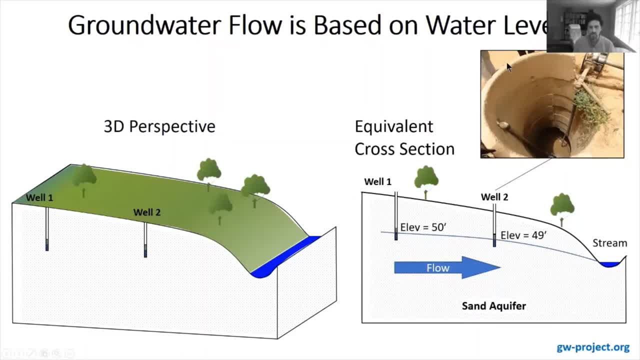 and that, essentially, is equivalent to what we're seeing in this well. This is a very large borehole, You know this is not something you typically see, let's say in the US wells used for irrigation or municipal water supply. 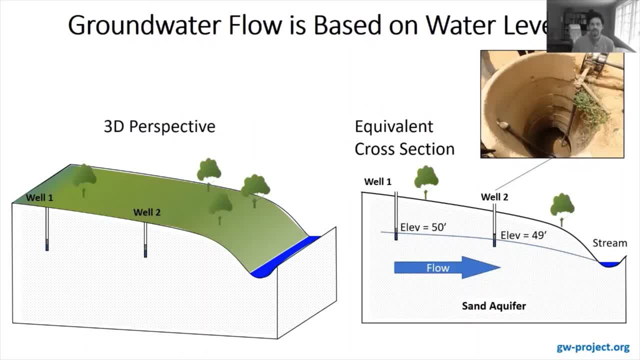 This, I believe, is in sub-Saharan Africa. This is probably- I don't know- two and a half foot diameter, But you can see here at the bottom this water. That water corresponds to the water that you see at the bottom of this well. 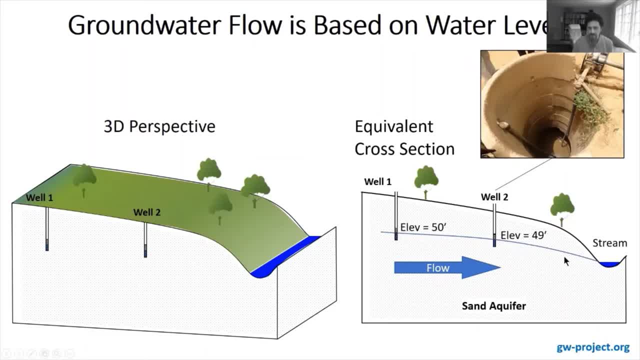 And that water defines the top of this aquifer, and this line then is the water table. Now the flow direction is based on the water level elevations. Here it's going from 50 to 49.. Therefore, groundwater is flowing in this direction. 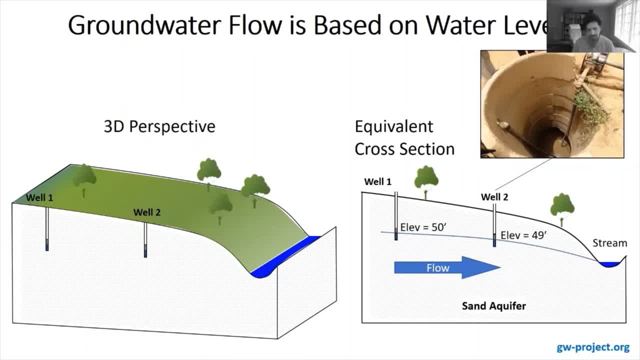 Essentially, we're talking about hydraulics here, right? We're talking about water flowing from a place of higher potential energy to lower potential energy, just driven by gravity. Okay, and there are all kinds of ways to describe this, and it's different when you're in soils above the water table. 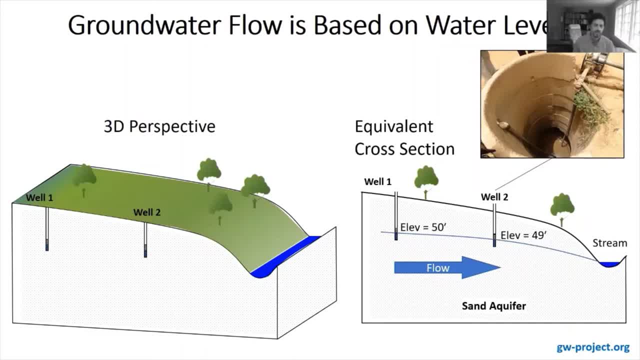 The bottom line is the takeaway I think should be: The groundwater flows in the direction defined by water levels in these monitoring wells. Okay, and when you have a lower water level, also called the hydraulic head, it's going to flow in that direction. 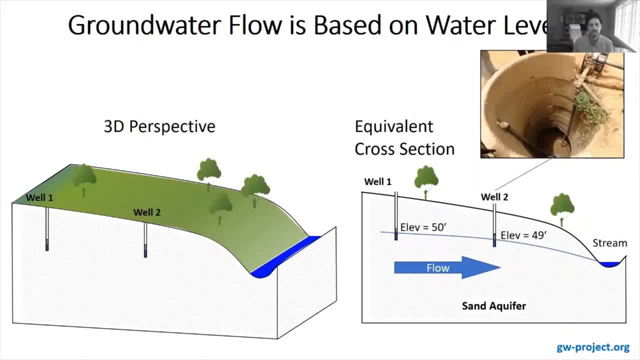 Now I've shown a really simplified case here. Generally, you need at least three points or three wells to define the flow direction. Nevertheless, this gives you the fundamentals. Again, go to this website here if you want some more detailed information. 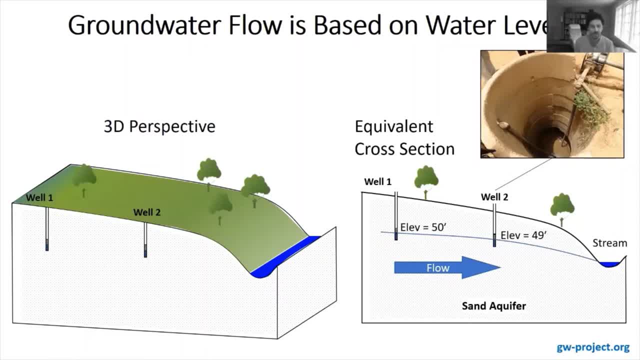 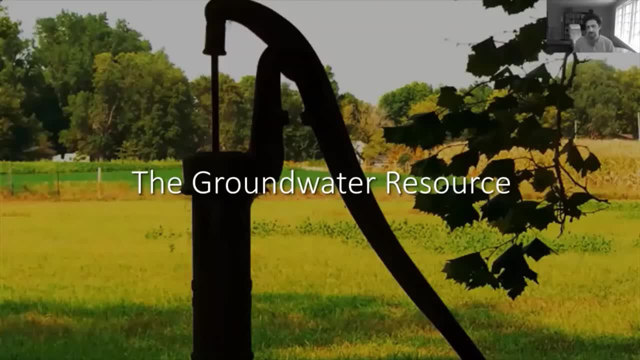 A better understanding, but a visual understanding of groundwater hydraulics. Okay, so those are the basics: Aquifers, aquitards, unconfined aquifers, water table and wells and hydraulic head and so forth. Let's talk about the groundwater resource. 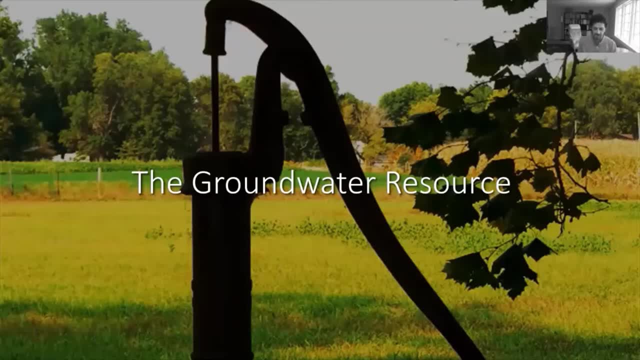 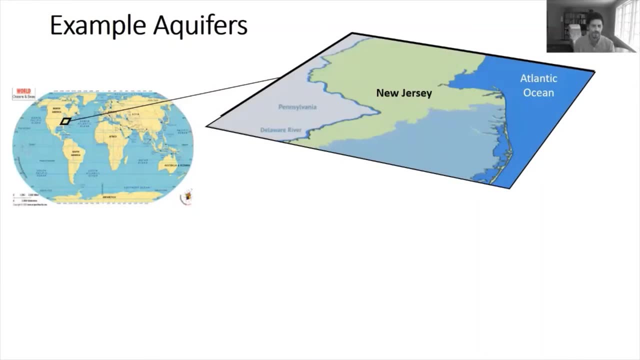 And I think for those of you who are not familiar with groundwater, this might be quite surprising. Okay, so here's some. We gave some example or simple schematics of aquifers. Let's look at some actual examples Here. we're taking a look at New Jersey, right? 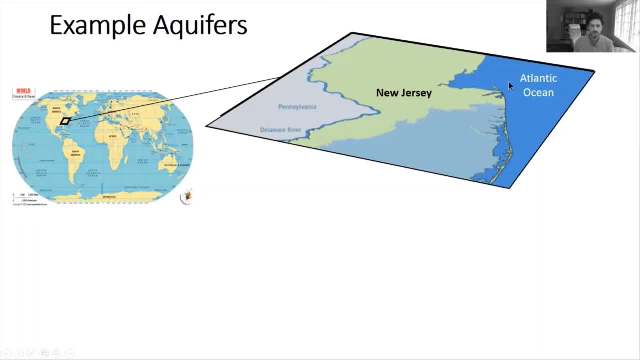 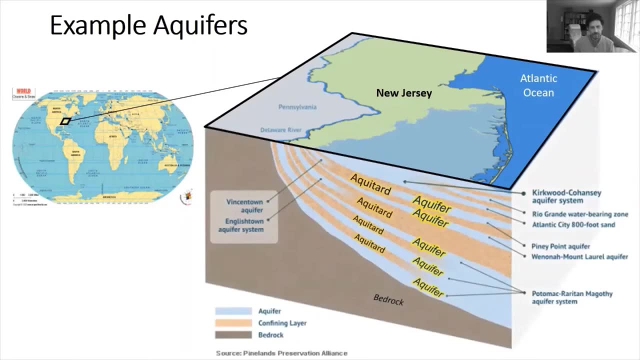 We're in eastern US, We're doing a little blow-up of New Jersey, Atlantic Ocean, Pennsylvania. If we look at a slice- right geologic slice- essentially what you see is that there's a sequence, an alternating sequence of aquifers and aquitards. 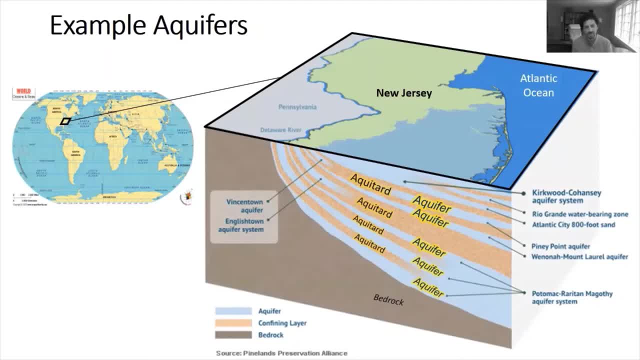 Okay, so this is water. This is a resource at depth. In this case, in this location, we're talking about 800 feet beneath the surface. Keep in mind there is quite a bit of vertical exaggeration in this figure, but nevertheless we are talking about 800 feet. 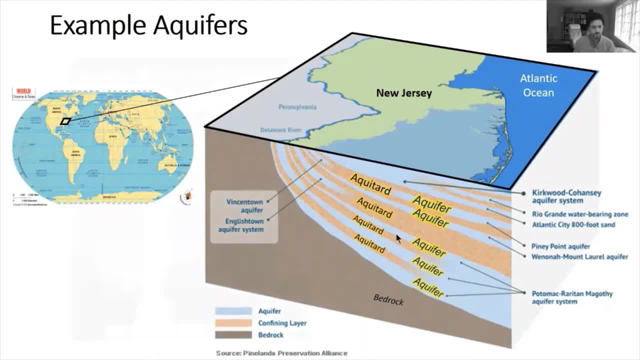 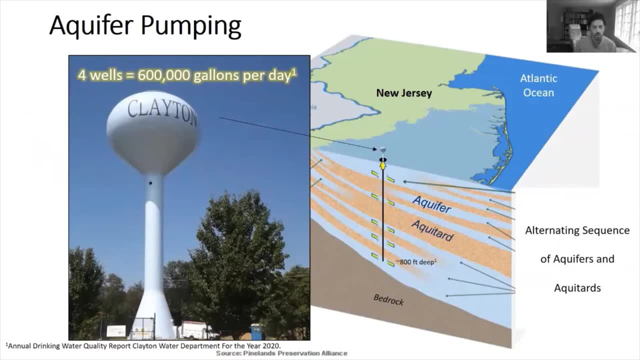 So aquifers separated by aquitards, And those aquifers are then the sources for groundwater which is pumped for municipal water irrigation, Also private wells. but take a look at this: for example, we've got an 800-foot well. 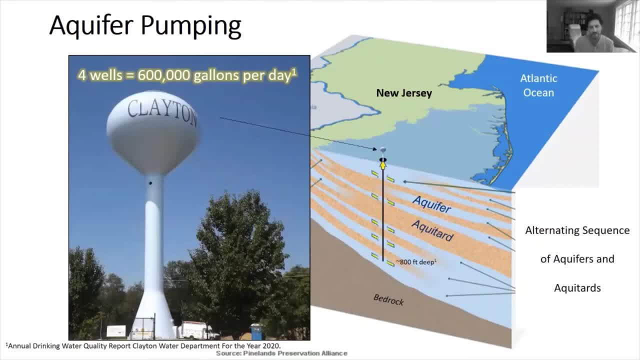 That's for the town of Clayton, And in many areas each town has their own system of pumping wells and water towers like this. In this one town- not a very big town- we've got four wells pumping at 600,000 gallons per day. 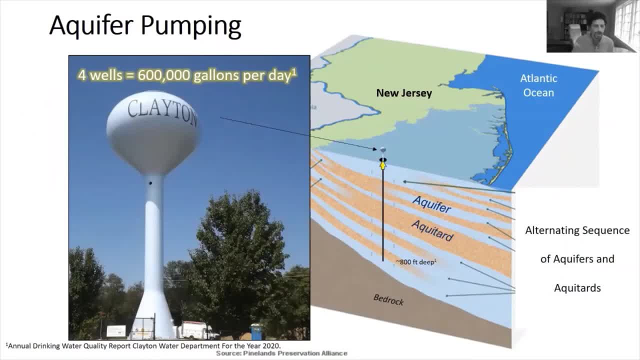 And, of course, essentially the whole town is relying on this water. It's all coming from the aquifer, It's all coming, it's all groundwater. There's no water, There's no surface water, It's not coming from lakes. 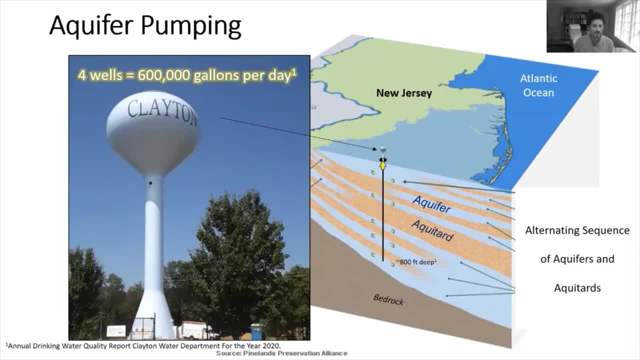 The groundwater is really, or aquifers, are the main reservoirs for water that we, or fresh water that we use, And you can see here just depicting the flow migrating really inward to this well, being pumped upward and then stored in water tower. 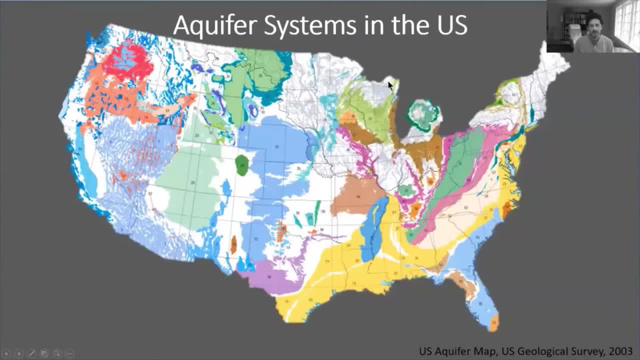 So that's just a little a piece of New Jersey. But we've got aquifers all over the US And the colored areas here are the major quipers supplying much of the water. But also keep in mind even those white portions, those aren't- quote unquote- Major aquifers. 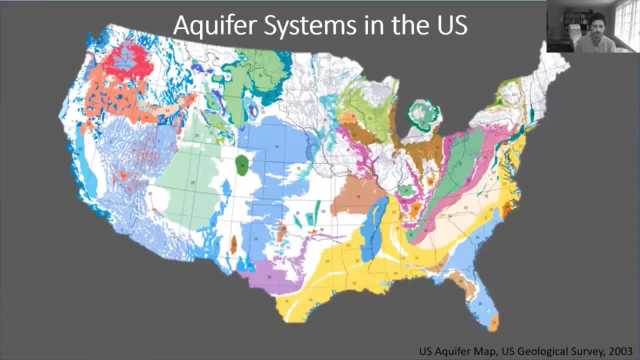 But there is significant groundwater. in those locations, for example, upstairs New York where I went to undergrad, you know essentially most of the water that is used municipally for municipal water and those locations, for example, upstate New York where I went to undergrad. You know essentially most of the water that is used municipally: municipal water, a game or water and drinking water. I guess expressions are not going to play you. it's very, very difficult to do And this is not going to work, but I'm goosebumps right now. 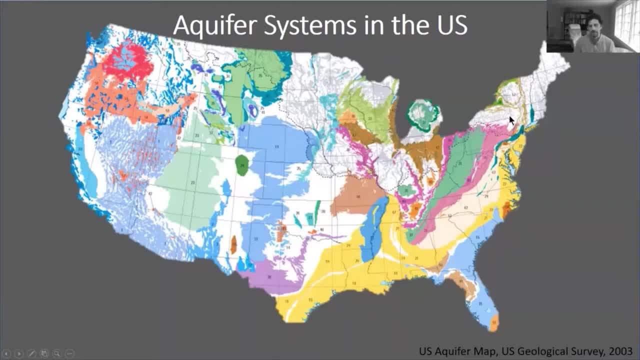 But I can. I can not imagine what it would have been done in 10 years or less. supply is actually a pump from um, from aquifers in that area, so there may not be major areas, but most of the us people are tapping groundwater and, quite unbelievably, there are 16 million wells. 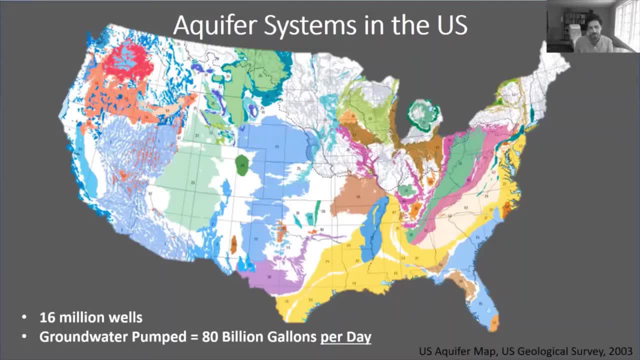 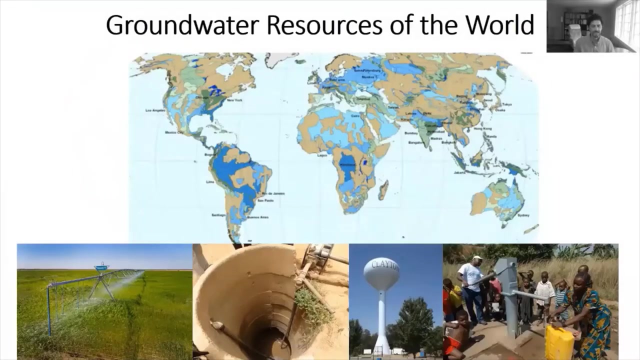 in the us, pumping a total of about 80 billion gallons per day. okay, that's per day and that's many, many times, uh, the amount that's flowing overnight in the fall. so it's pretty astonishing. we're really relying on groundwater. it's a major resource now also, that's the case. 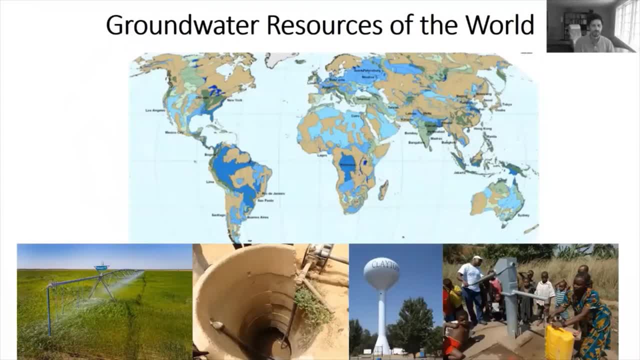 worldwide. okay, again, i'm showing this map- that the various blues, uh, represent major aquifers, but again, even though in those other regions- in this case the kind of light that's flowing around- they are also using groundwater. they're using it for irrigation, they're using it for municipal supply, they're using it for, you know, small town or community. 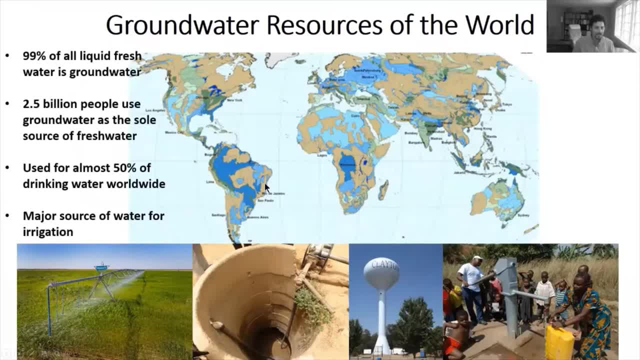 fresh water. 99 of all liquid fresh water is groundwater. two and a half billion people use groundwater as the sole source of fresh water and used it's used for almost 50 percent of drinking water worldwide. so clearly this is a major source uh for groundwater in this and also a major source for irrigation. 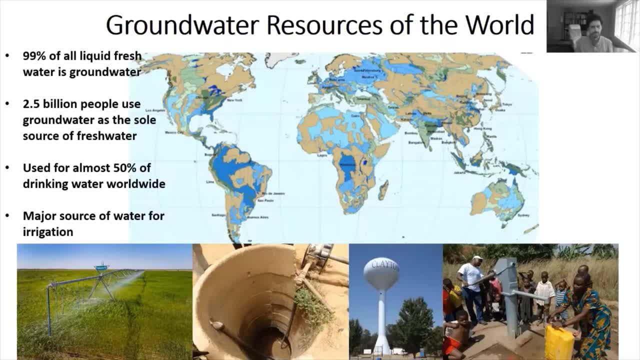 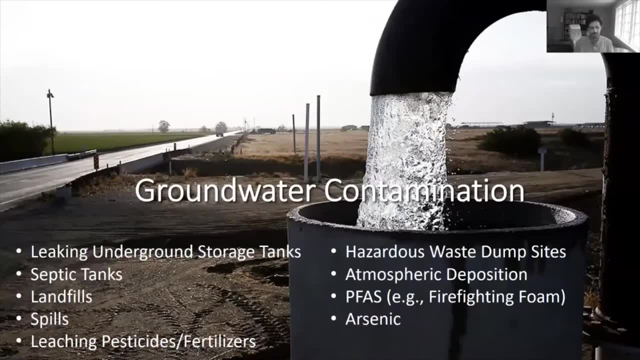 so we're really depending on this resource. however, it's, in some areas, highly contaminated, and it's contaminated for a number of reasons. i've just posted about nine here, but there are many others. we're talking about leaking underground storage tanks, septic tanks, landfills that don't have liners. 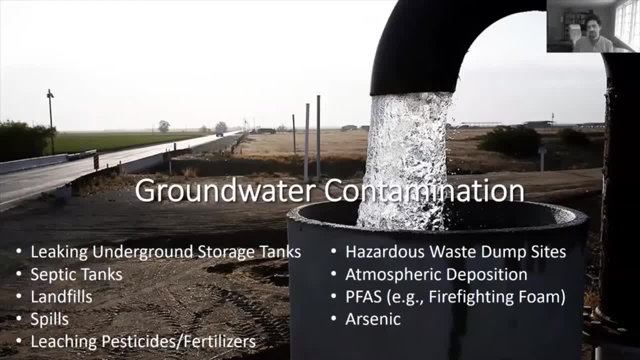 and there are many of them: spills of solvents and petroleum products or dissolved metals at old manufacturing facilities. we have leaching pesticides, that's widespread hazardous waste dump sites. we're talking about areas where drums of hazardous waste in the thousands have been buried and are leaching and creating groundwater contamination. you've atmospheric deposition in the 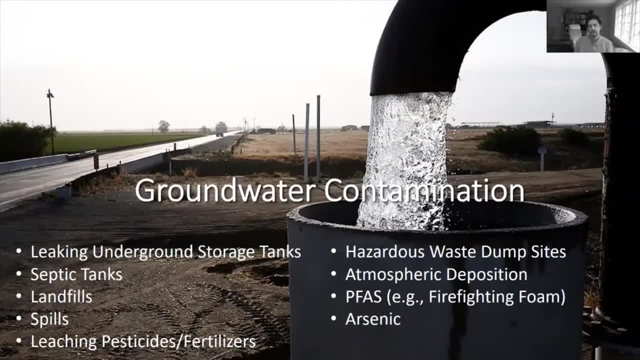 ground and then subsequent leaching into the groundwater. i'm going to show an example of a contaminant referred to as pfess. in this case, i'm going to show a firefighting foam- pfess, you may have heard in the news. it's a very hot topic. it's, it's probably the- the groundwater. 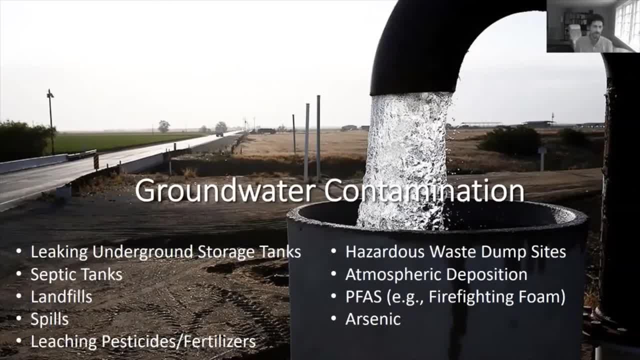 contaminant that's focused on most right now and i, as i would like to tell you- you'll hear a lot about it, you'll hear how it is this. i'm not really here to talk about toxicology, but i would say, be be careful about believing all the news you know regarding how dangerous this stuff is, and 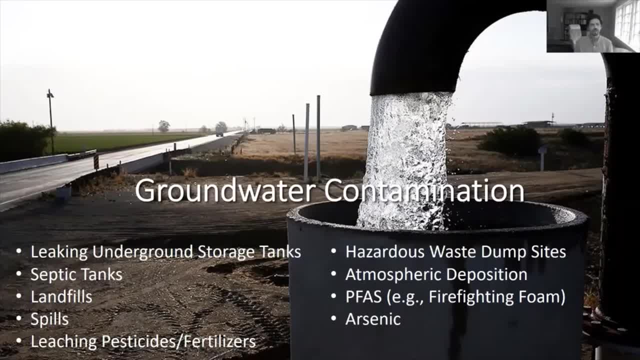 and the the um, what concentrations are acceptable in water? so i just wanted to say that there's a lot, there's a lot of fear news out there. just be careful, okay. so contamination, groundwater contamination- now the first thing we need to do in order to get wrap our 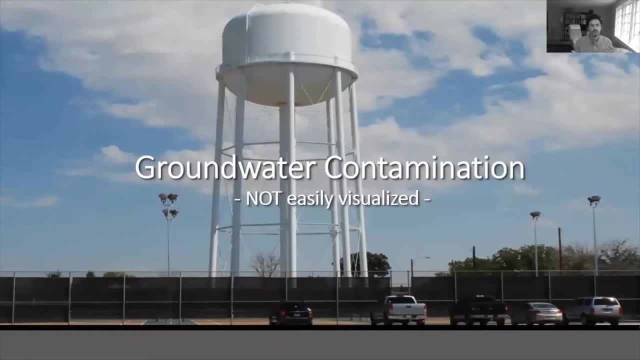 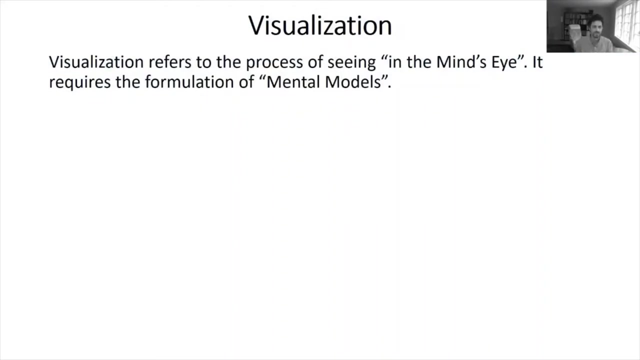 head around. this is to be able to visualize groundwater contamination, and it's not easily visualized because it's hidden, right, it's bleeding, it's beneath the surface. so one thing we want to do is get a better, and this is part of really the focus of this presentation- is to get a better. 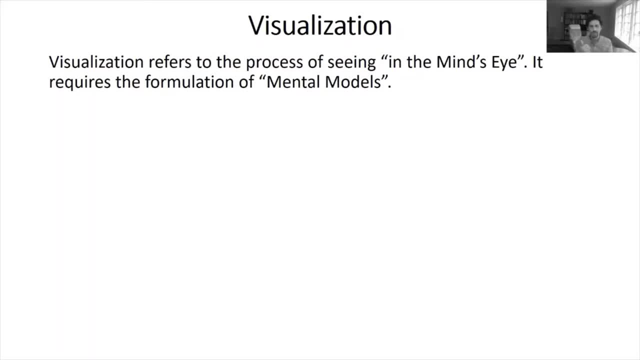 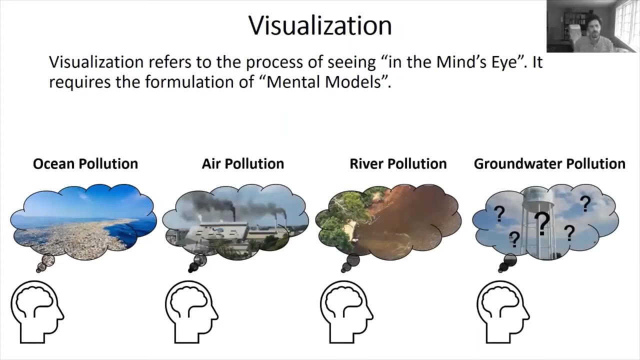 uh, build our ability to visualize in the mind's eye, in the mind's eye, what we're talking about with regard to groundwater contamination. so when i'm talking about visualization in this context, i'm not talking about computer animation or computer simulation or anything like that 3d modeling. i'm really talking about the mental. 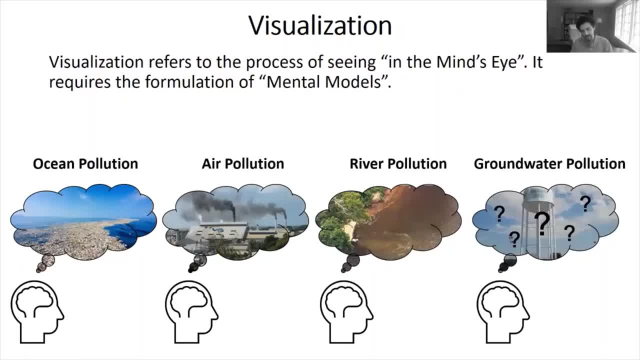 model when you close your eyes and you think about a particular uh contamination scenario. you have that you kind of you can visualize it. so in the case of ocean pollution, we can clearly. we clearly have a mental model, same with air pollution, river pollution, but with regard to ground. 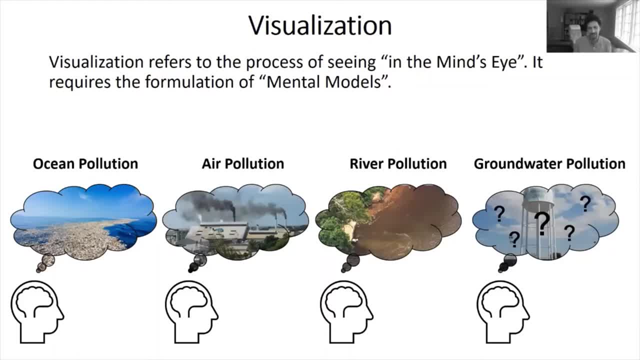 water pollution. it's hidden, it's difficult to visualize, and that's one of the focuses of this presentation and one hopefully you're going to come away with this with some a better- uh, a better- mental model about groundwater contamination. so one way to do that is to 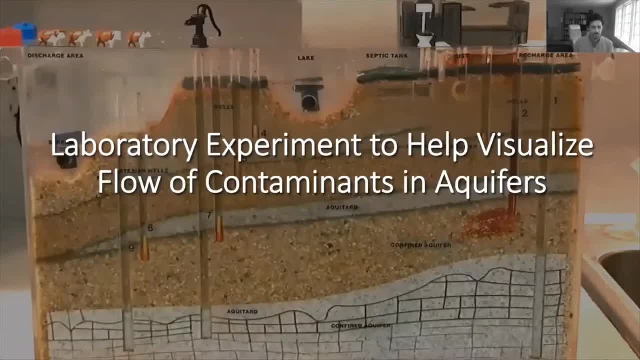 first look at a laboratory experiment. okay, this is on the order of what? maybe a foot and a half, two feet wide. it's a laboratory experiment and it's developed to help visualize the flow of contaminants. okay, actually, to look at the flow and transport mechanisms. so we're talking about a water saturated sand tank. 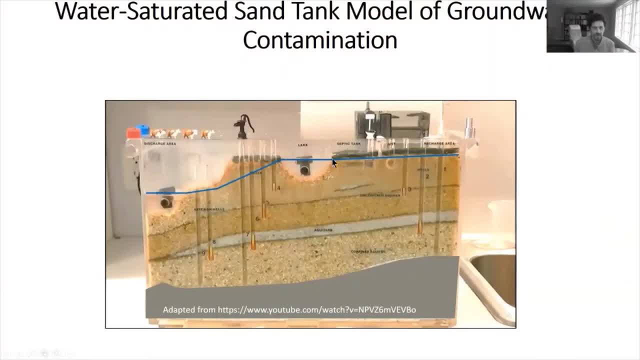 okay, and you can see this blue line is essentially that water table that i was talking about. so everything, beneath all of the sand, beneath this water, beneath this blue line, is saturated, and you can see the gradient of this blue line right. the water table is higher here than it is. 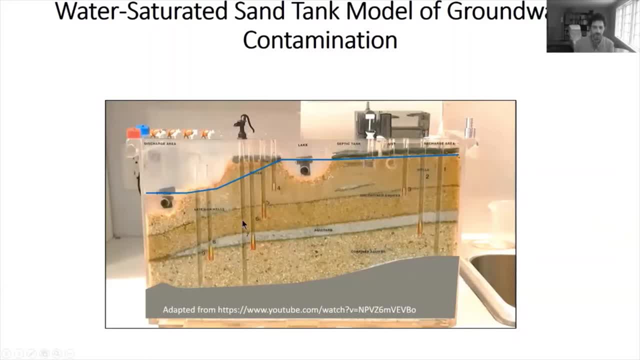 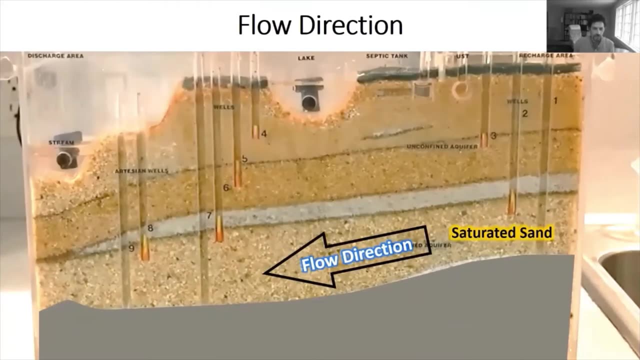 here and here. therefore, water is flowing to the left. okay, we have an aquitard here, another aquitard down here and this is our confined aquifer, okay, so we're going to focus on that. so, again, we have the saturated sand. i've already defined the flow direction. 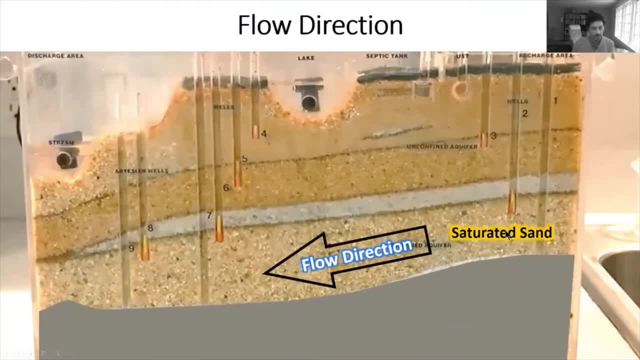 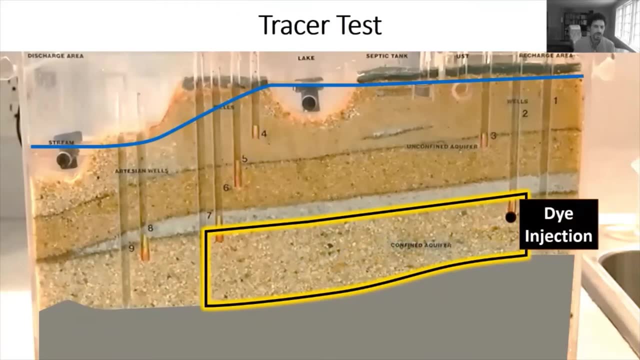 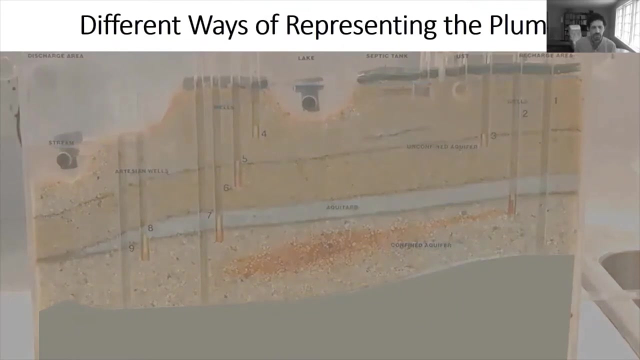 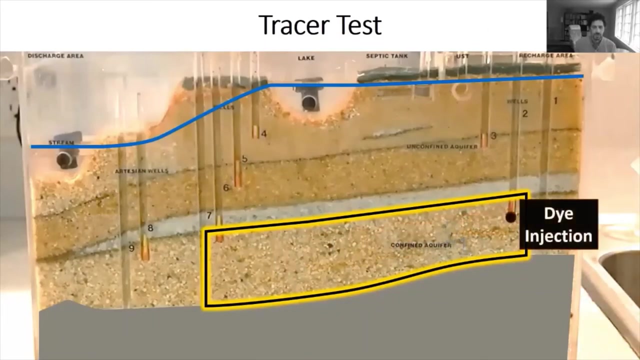 it's from right to left, based on the water levels. uh, based on the water table elevation. let's consider this dye injection. okay, the dye injection would be analogous to, let's say, a con, a continuous asant quantity or water composition of the phenol. somehow are different time intervals like this. i'm just labeling this: t one through t4. this could be on the order of hours, minutes it's. it's depends on the permeability of the sand and also of the hydraulic rating. let's take a look at this one more time just to get a good visual. okay, we're injecting the dye. groundwork meter: proceso-itals e-list. 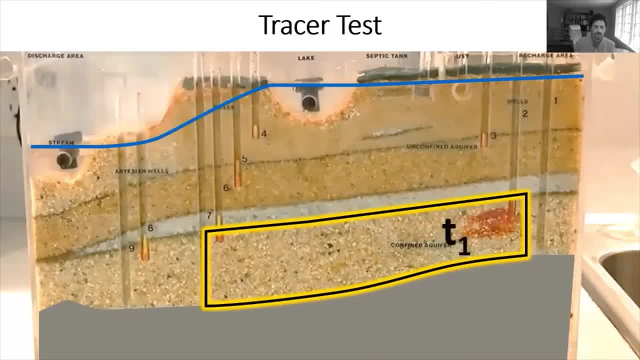 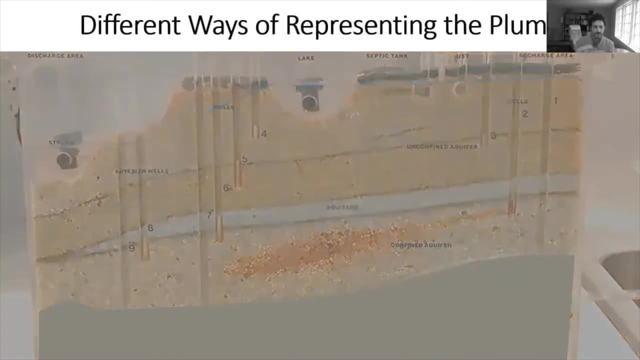 is flowing, that plume, so to speak, is advecting in the direction of flow, and it's also just, it's uh, it's dispersing right, lateral, laterally and also vertically, and that's a function of this, this solute basically making its way around the sand grains. okay, now there are a couple where you don't. 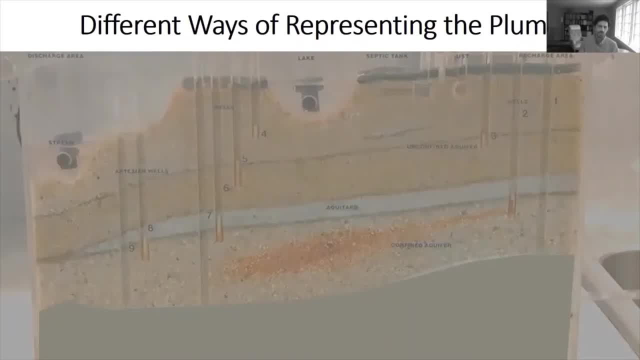 obviously see that in the subsurface. in reality, what we usually do, or what we do, is we collect samples from wells, we measure the concentration, we plot it up and we define what these distribution of contaminants look like. and there are a couple of ways to do that. one is to denote the 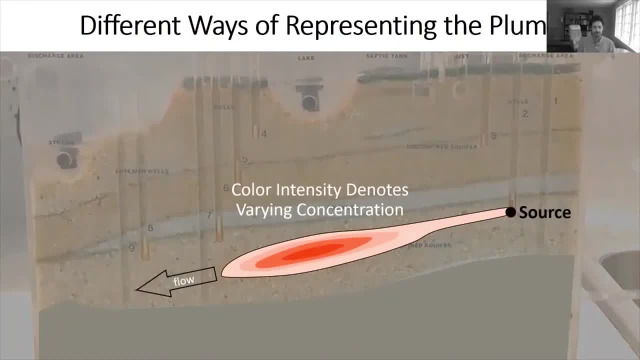 concentration variability with different colors. okay, that's one way to represent it. another way is to give it different colors, right. so the blue, the light blue, would be lower concentrations, the red would be the highest concentrations. and you can see here that red is right at the center of the sample and the blue is at the bottom of the sample and the blue is at the 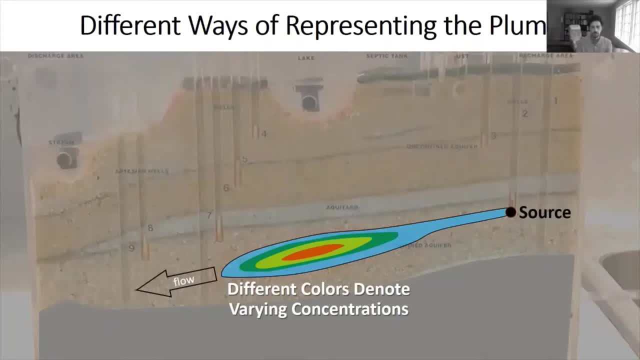 center of the sample and the red is at the center of the sample and the blue is at the center of of the plume. Or we can denote it just with a single color, which would represent the full extent of the plume. And I'm showing you this because I'm going to use these kind of 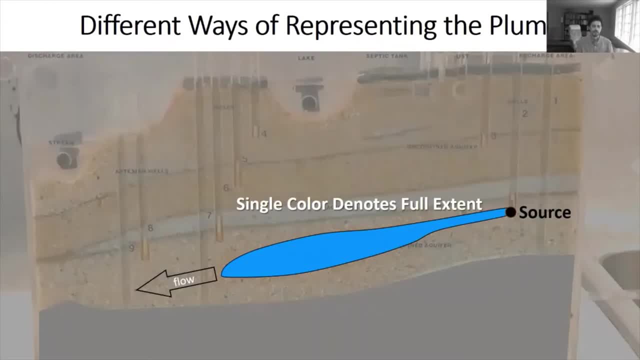 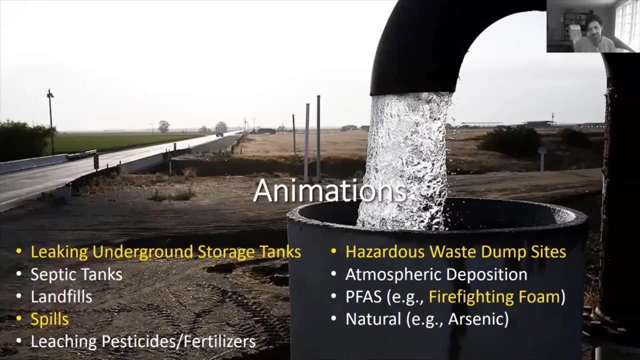 representations in subsequent animations. So the idea of these. I'm going to show you some animations- One is hypothetical- just to show you some of the basic mechanisms of groundwater contamination, but also some animations that are based on real sites, actually contaminated sites that we characterize, we run out, we define the geologic materials, the distribution of 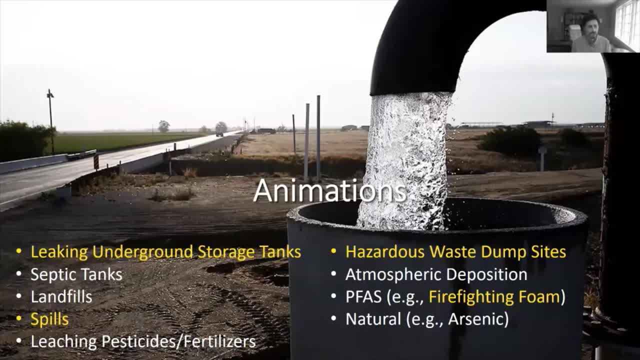 contaminants by sampling, monitoring wells, the likely location of sources And what I'm going to show you in particular: an example of leaking underground storage tanks, spills, hazardous waste dump sites and also the sampling sample with firefighting foam. Okay, so that's what I'll take you through. 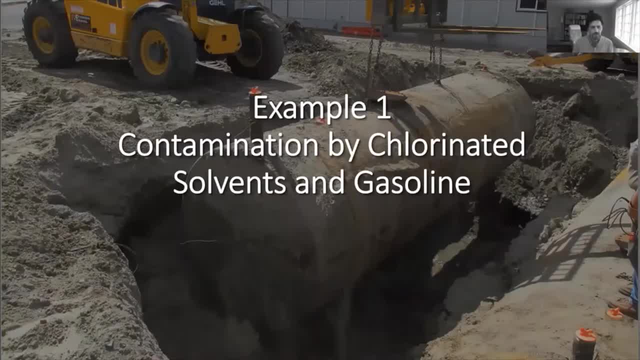 Okay, the first example is contamination by chlorinated solvents and gasoline. This picture in the background is an underground storage tank at a gasoline station. This is typically what you have: 10,000 gallon tank, 20,000 gallon tank. Historically, these tanks were rusted. 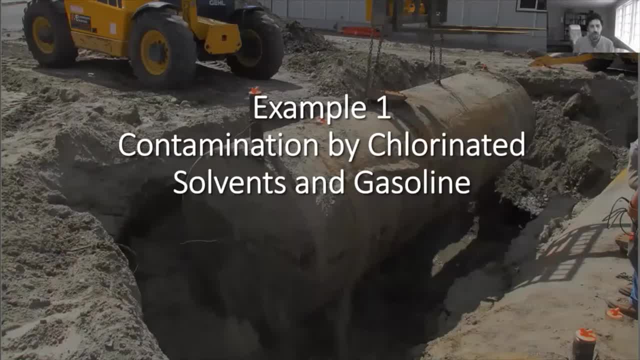 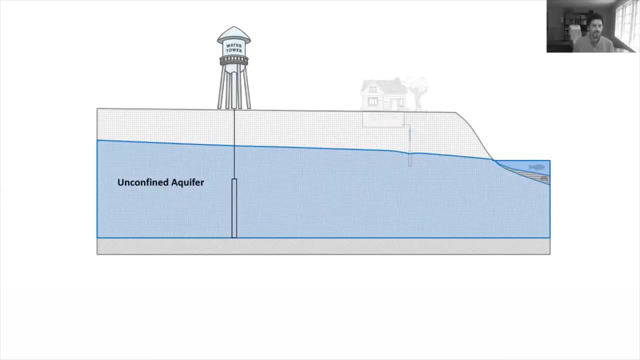 and you had liquid gasoline just by migrating downward and hitting the water table, Okay. And also you have a scenario where you'd have liquid solvents from old manufacturing facilities where they're using solvents to clean metals, for example. So let's look at a simple case here. unconfined aquifer- Again, we know the groundwater. 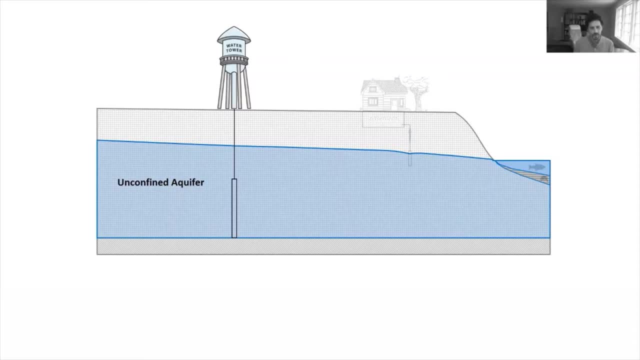 is flowing from left to right, based on the water table and the gradient. Consider this, this municipal water supply. it's pumping water is flowing. we're able to see the water is flowing inward towards the screen portion of that well And that sucking action is going to create a 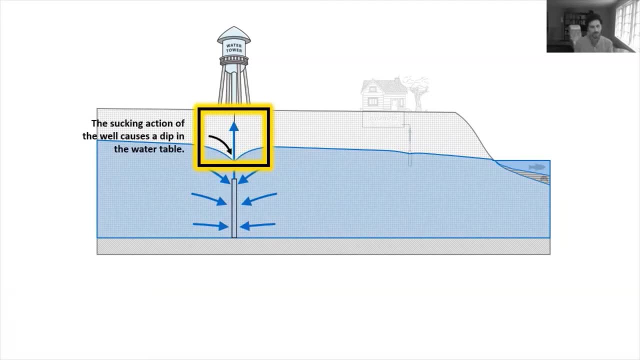 depression, a dip in the water table. That should kind of be intuitively obvious, right? It's like you have a bathtub, you open the plug, the water drains and it drains basically of a cone of depression. In this case it's kind of like a drain, except we're actually pumping. So this 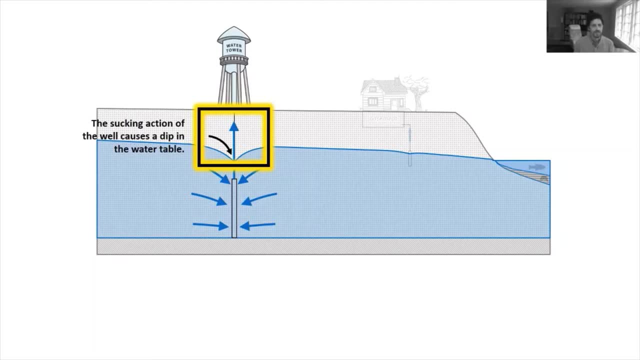 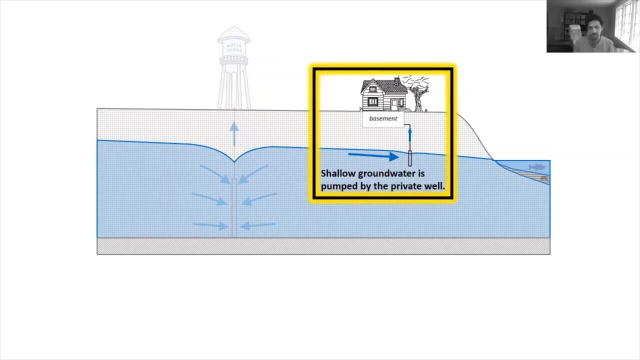 is called a cone of depression. This is a key feature. Now take a look at down gradient. We've got a shallow well just for private use And that water is. it's just the shallow water that's being pumped Deeper down. the groundwater is actually discharging to surface water. okay, And 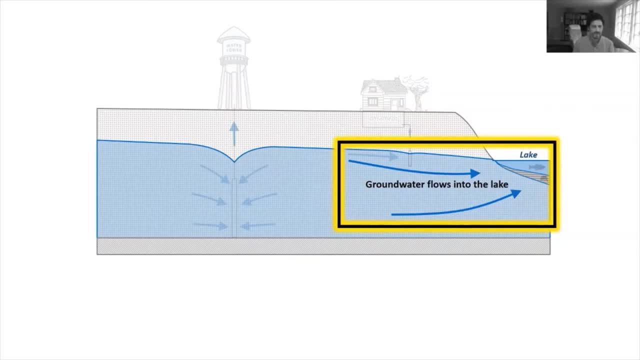 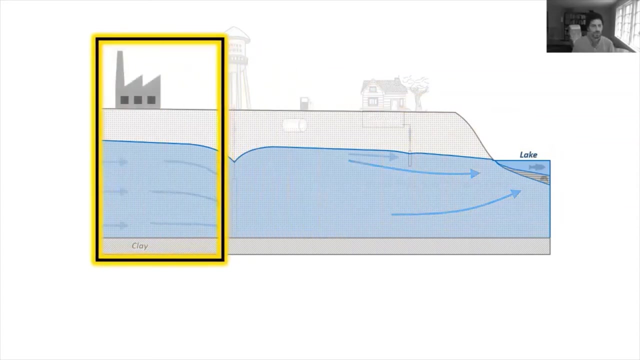 that's. that's that's important, because it essentially it indicates that there are cases where you can have groundwater plumes that not only impact private wells but also will discharge to surface water bodies and could affect the ecosystem, And that's what we'll show in just a second. So consider this scenario. 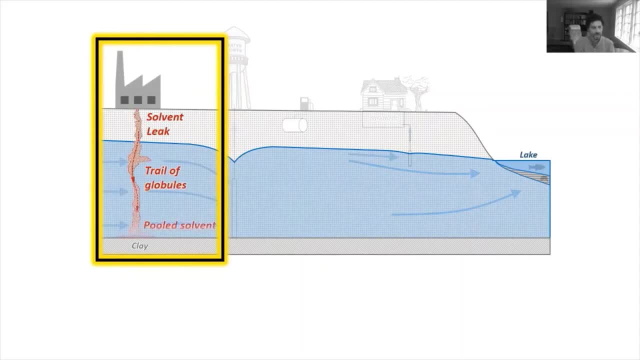 here, An old factory. you had a solvent leak. This solvent is. it's a liquid solvent. Okay, the solvent is heavy, It's heavier than water, so it makes its way. it hits the saturated zone, it hits the aquifer and it continues to sink And it leaves behind a trail of globules. 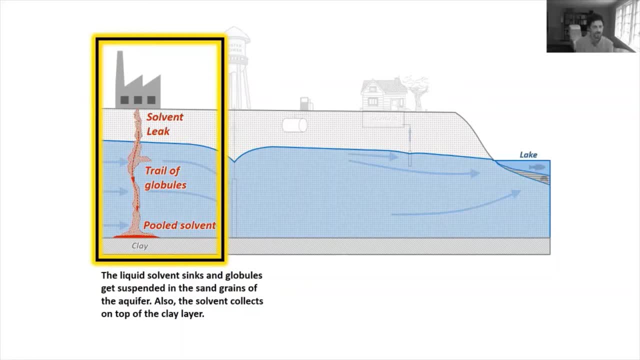 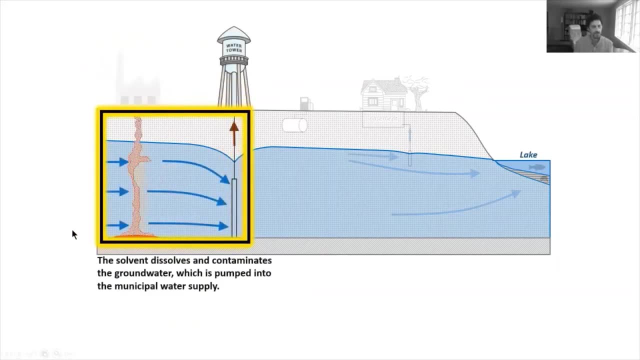 kind of liquid globules that get stuck in the sand grains, And also it can pool on the surface here of lower permeability units. Okay, so what happens? The groundwater is flowing. this is essentially clean groundwater, fresh groundwater. It migrates through this zone of 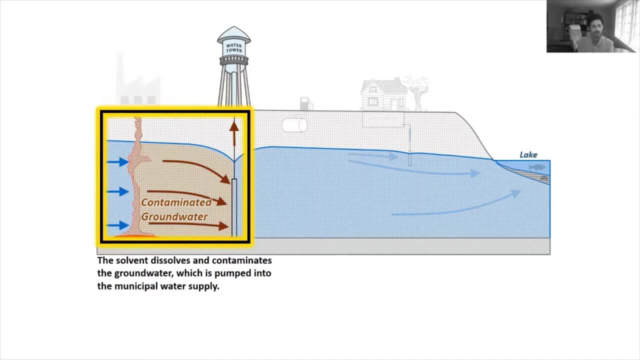 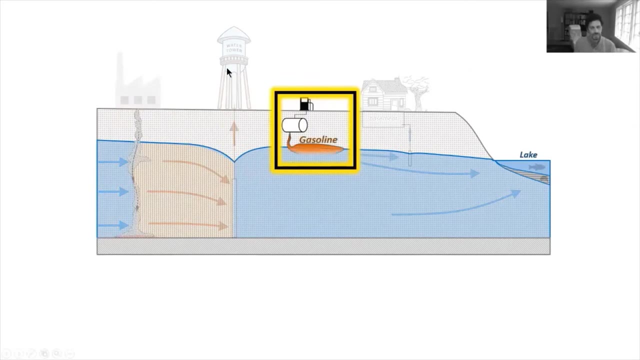 liquid, liquid, liquid chemicals, which then dissolve and, as a result, you have a groundwater contamination plume and that's making its way then to the municipal water supply. Another scenario is this underground storage tank. so you have a leaking underground storage. 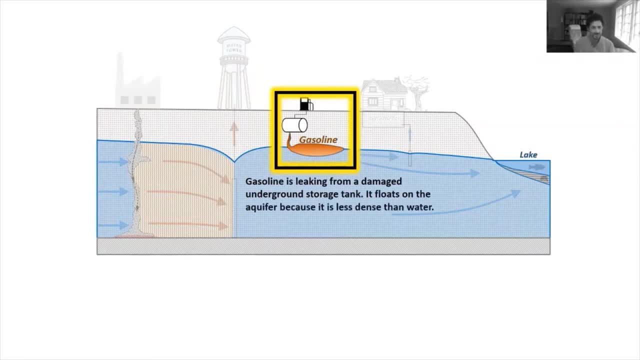 tank. In this case, the liquid that's leaching is lighter than water, so it doesn't continue to penetrate. Instead, it essentially floats on top of the water table. This is a schematic. It's a little bit more sophisticated, if you will, but for all practical purposes it's. 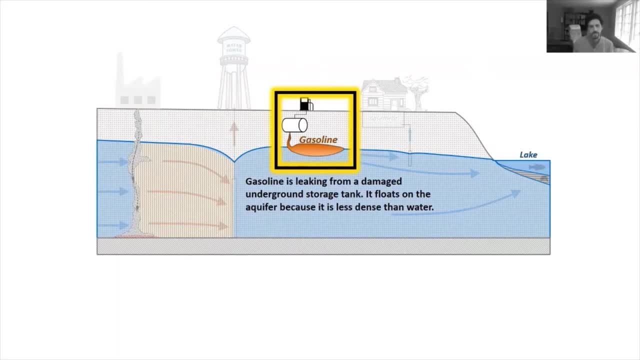 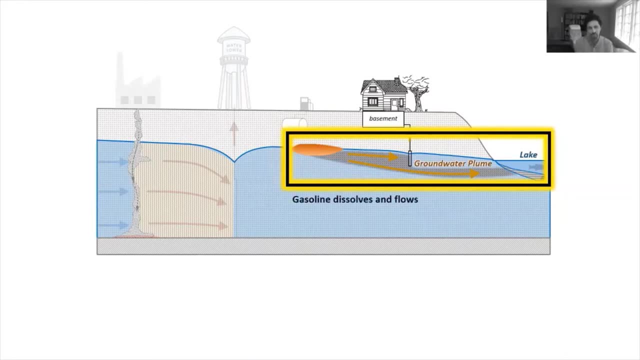 essentially floating on top of the saturated zone. Similarly, water is migrating past that and around that liquid contaminant. It's dissolving and you have a groundwater plume that's migrating, downgrading. In this case, the groundwater contaminants are being pumped by the private well, so we've 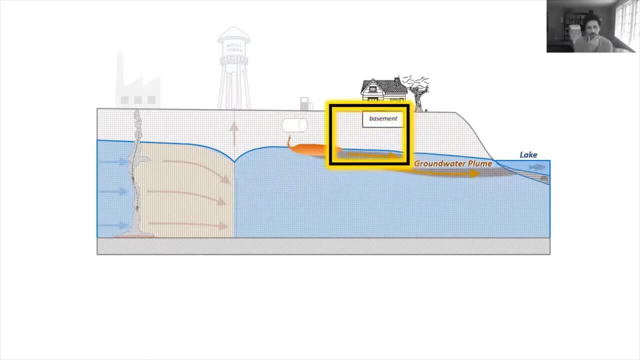 got an issue there And also we've got this issue of what's called vapor intrusion. Here's a basement, There are cracks in the basement, There are some pump. You have basically pathways beneath the basement into that living space. There are two things going on here. 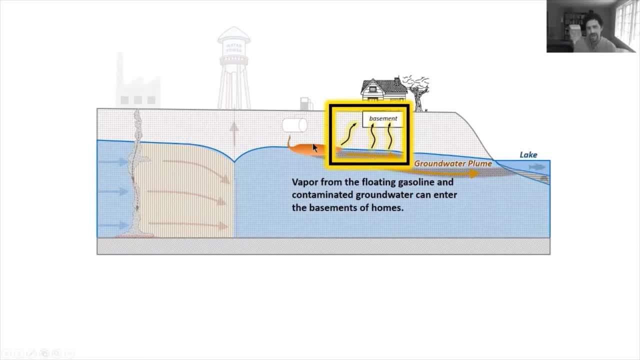 You can have vaporization of the actual gasoline, so you have vapors migrating towards the basement, and then you can also have volatilization of the chemicals that are dissolved in the plume. So really there are two mechanisms by which that air in the basement can become contaminated. 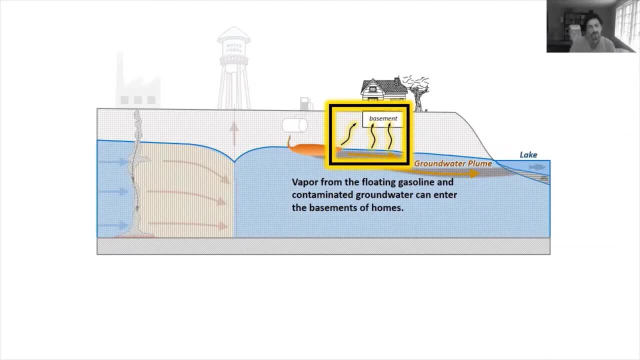 It's just an artifact of actually a leaking tank, whatever. It could be hundreds of feet away. So it's not directly in the basement, It's just an artifact of actually a leaking tank, whatever. It could be hundreds of feet away. 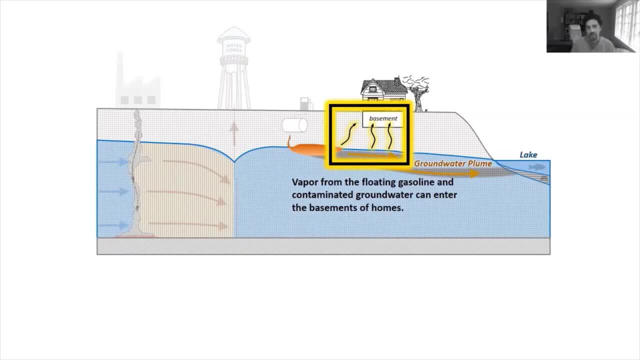 So it's not directly in the basement. It's just an artifact of actually a leaking tank, whatever. So it's not directly in the basement. So it's not directly in the basement. So it's not directly in the basement, But in fact there is an air quality issue now. 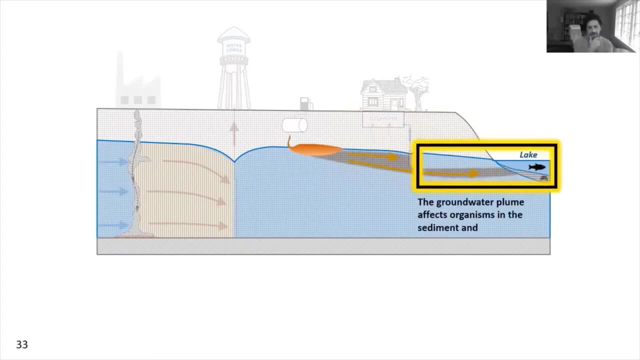 And also you have, like I said previously, that groundwater plume is now discharging the surface water. That could be affecting benthic organisms which are basically the basis, the bottom feeders or the bottom of the food chain, So that can result in contamination of the higher order organisms. 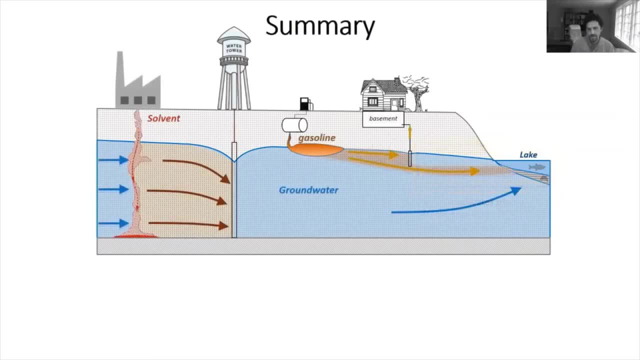 Okay, So here's a summary Again. the solvent: this is a dense solvent, liquid solvent, This is called dense non-equal phase liquid. It leaves globules, It pools. The groundwater flows through that zone. It becomes contaminated. 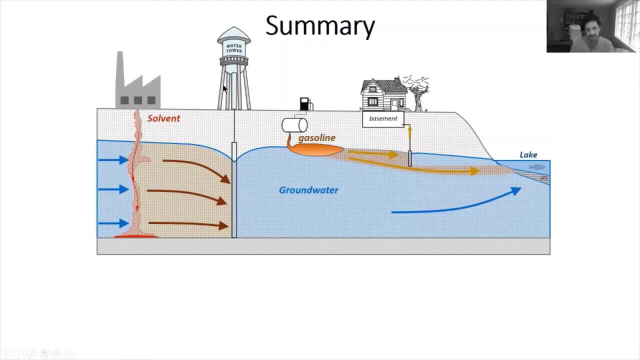 That's then pumped into the municipal water supply, You've obviously got a groundwater issue for the community Also leaking underground storage tanks. The gasoline is less dense than water. It flows through a hole Or an air jet Right on top of the saturated zone, basically at the water table. Similar to the solvent, it's. 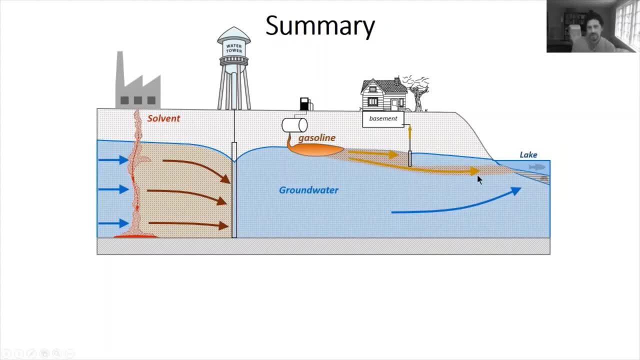 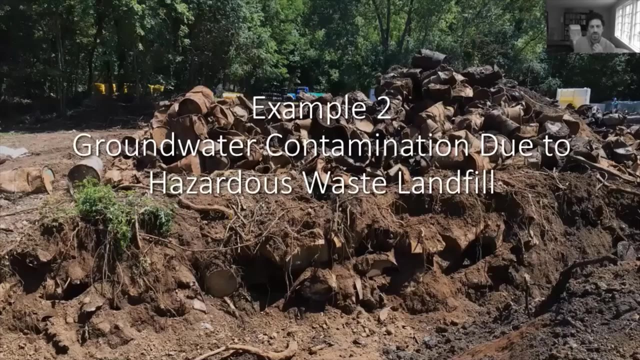 essentially liquid chemical that dissolves, You have a resultant groundwater plume, makes its way to the private well and also affects surface water quality. Okay, let's look at another example based on a real site. Wow, time's gone by. Okay, this is a groundwater contamination due to a hazardous 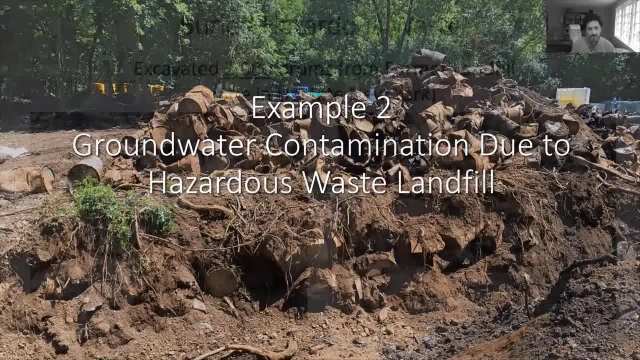 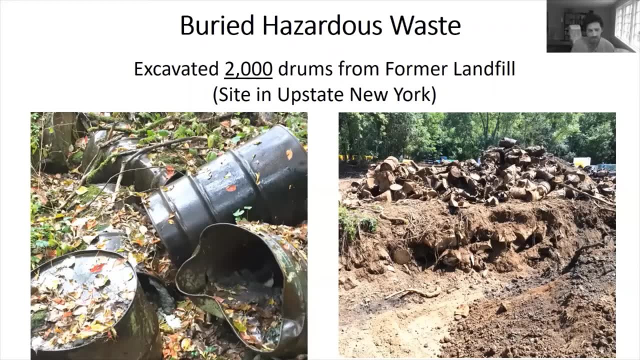 waste landfill. That's an actual picture. This is quite a surprise to me. This is just a project that was performed just a couple of years ago in upstate New York, where 2,000 drums of hazardous waste were found buried in a forested area. These are the kinds of sites that you heard. 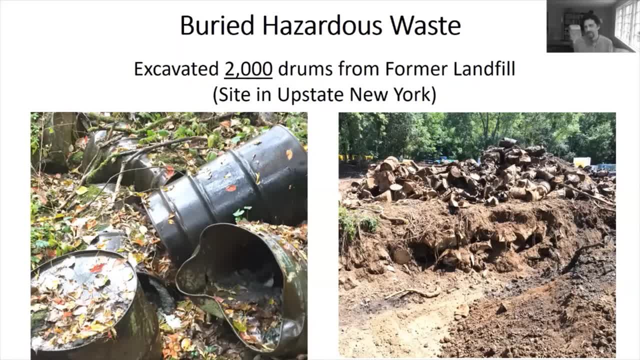 about in the 1980s. In 1990s I thought that they were all gone, but in fact they're still around. So they found all of these drums. They had liquid waste, they had a combination of solvents, They also had sludges. 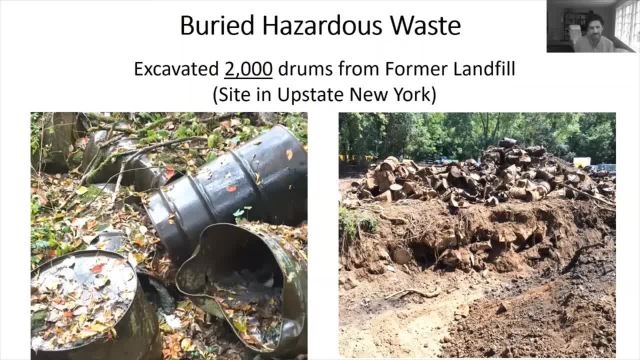 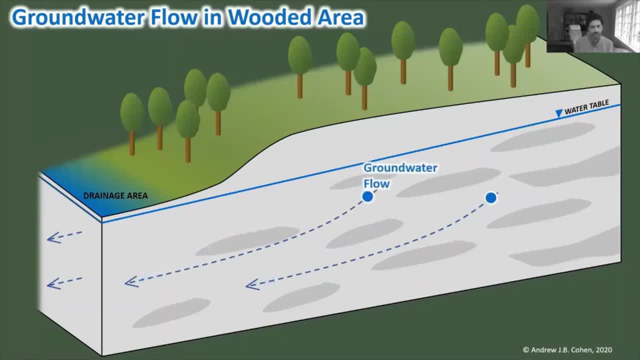 paint sludges and all this stuff is now leaching into the groundwater. Here's an oblique view. Essentially, this is a conceptual model of what's going on. You have groundwater flowing towards the left again, consistent with the declining elevation of the water table. 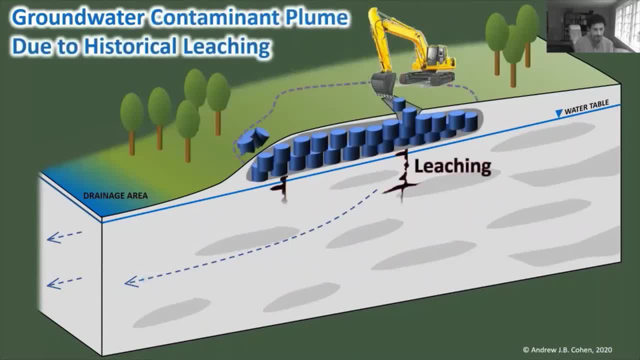 In that direction. they found 2,000 drums. Essentially, there are 2,000 drums that are leaking, and they're leaking these chemicals. Okay, and similar to the other scenario I pointed out. there's dissolution of that liquid chemical and then a resulting groundwater plume. Okay, 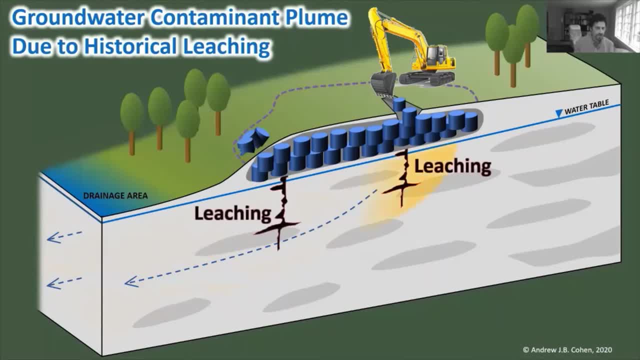 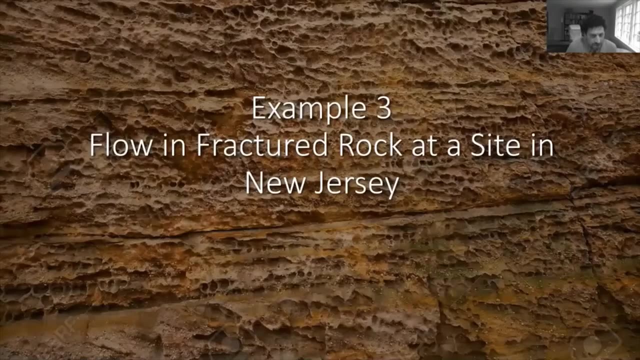 so let's look at that one more time. We've got leaching. We've then got groundwater moving through those zones. The contaminant is dissolving and you have a resulting groundwater plume migrating away from this. Let's look at flow in fractured rock. So I just essentially was just focusing on 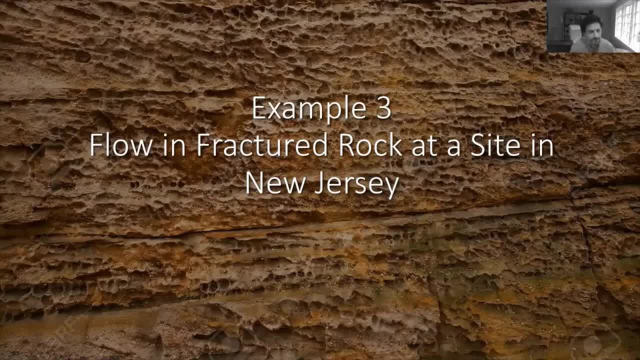 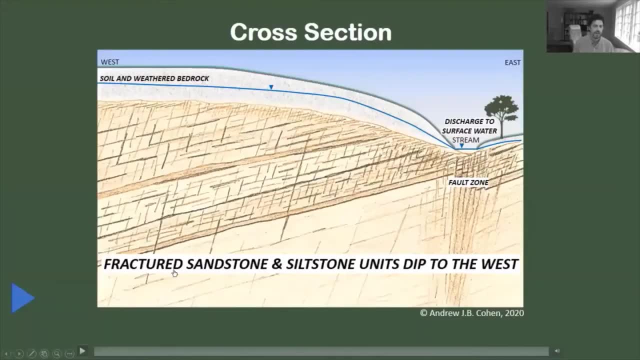 unconsolidated materials, alluvial materials, but also the same thing happens in bedrock, okay, in coarse bedrock. So here we're looking at a cross-section of a fractured sandstone and siltstone. We've got here's our bedrock, with these fractures, vertical fractures. 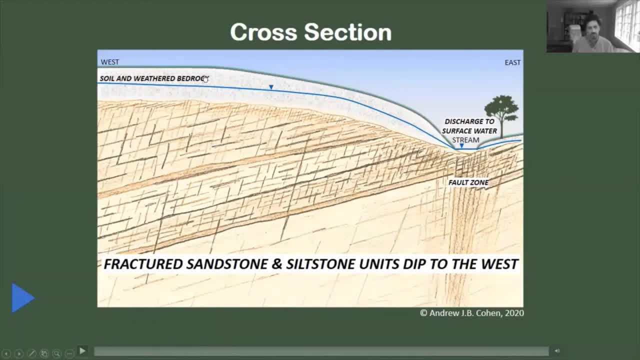 some of these fractures and then we've got a cross-section of a fractured sandstone and siltstone Horizontal fractures. We've got soil and weathered bedrock on top. This blue line denotes the water table. Therefore, flow is in general towards the right, although, as you'll see, it takes kind of. 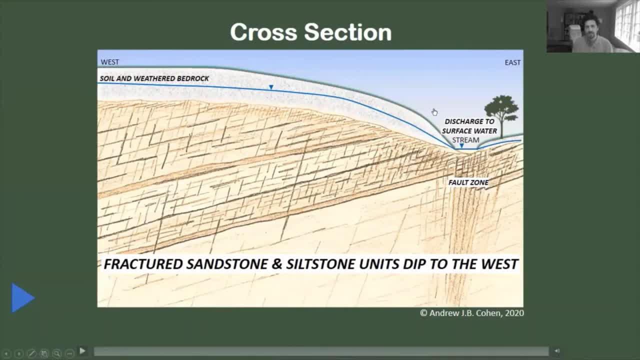 circuitous pathways and all of that's discharging to the surface water. This fold zone essentially also creates a preferential pathway or a high permeability pathway. Okay, so let's take a look at this. So again, we've got the bedrock. 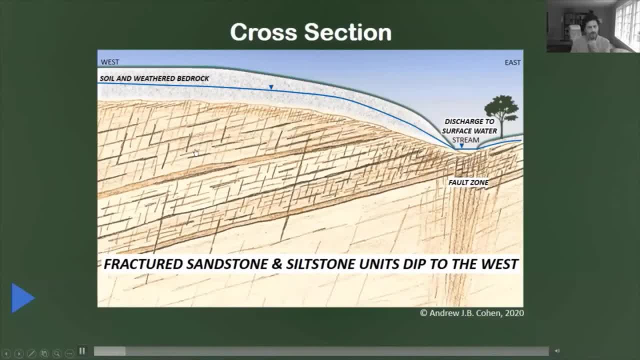 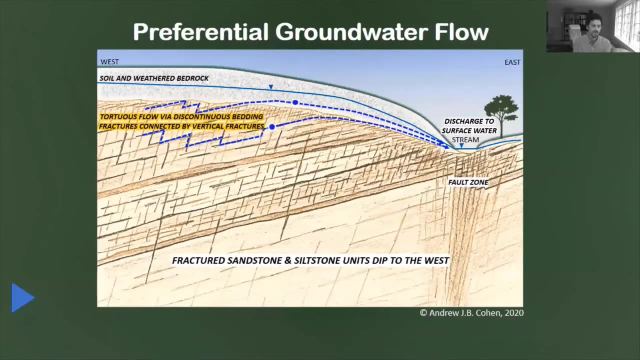 Vertical fractures. Some of them connect up to other fractures, but not all of them. Now, as a result of the discontinuous fractured pathways, groundwater is flowing in this kind of tortuous pattern. okay, and it's flowing, you'll see, generally slower than in some of the more. 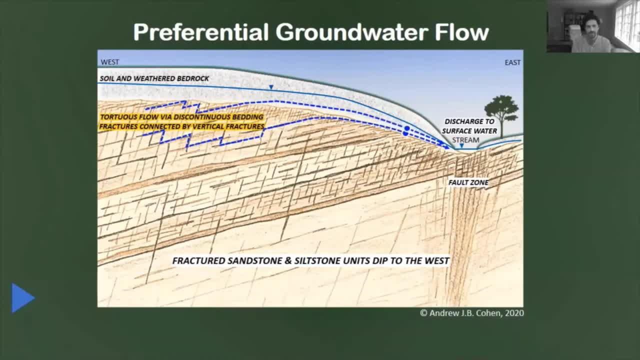 continuous fractures and it makes its way down over and discharges to the surface water body. Okay, in contrast to that- let's see we're getting there right- There are places where you have continuous open fractures for hundreds of feet. I mean, these are extremely fast pathways for groundwater flow. So, whereas 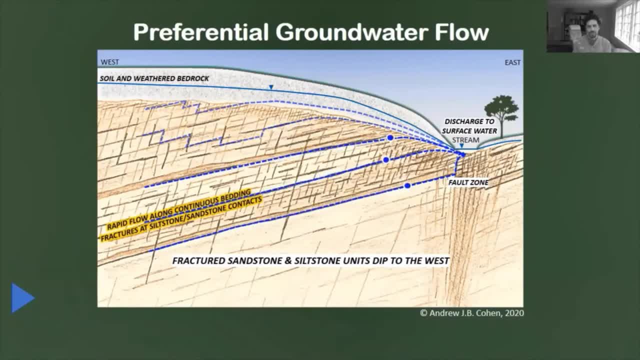 groundwater flow and unconsolidated materials might be on the order of 100 feet per year. these things are probably moving, you know. probably 100 feet, possibly 100 feet per day. So that was the pathway. So now at the top, here we've got a source. let me pause that a little bit. 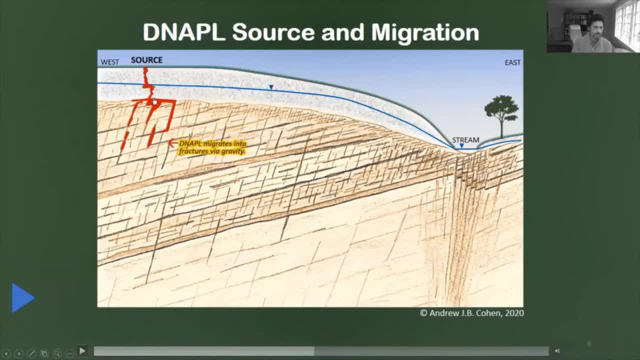 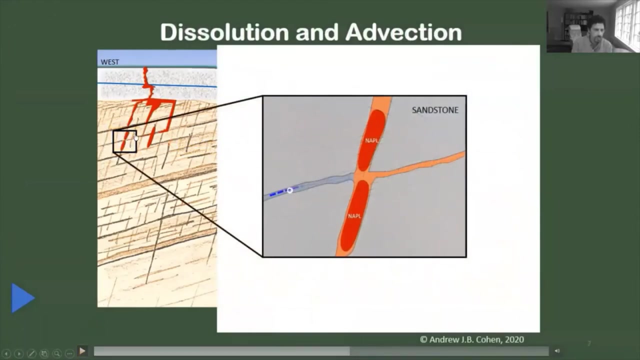 so here's our DNAPL source, right, our non-aqueous phase liquid source. It's heavier than water, makes its way beneath the water table and into the fracture network. the fracture network. Okay, now take a look at just a zoom-in of just a portion of the bedrock where you've 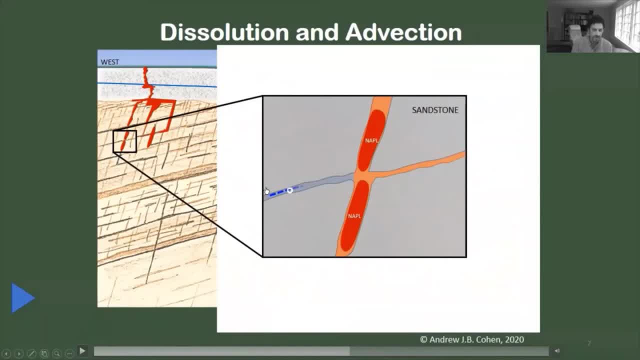 got a couple of these globules. Okay, so this is a zoom-in. So you've got this fracture, this fracture. here are some globules of the liquid waste- right, It's kind of trapped in these fractures. On this side, this circle represents essentially like a package of water. 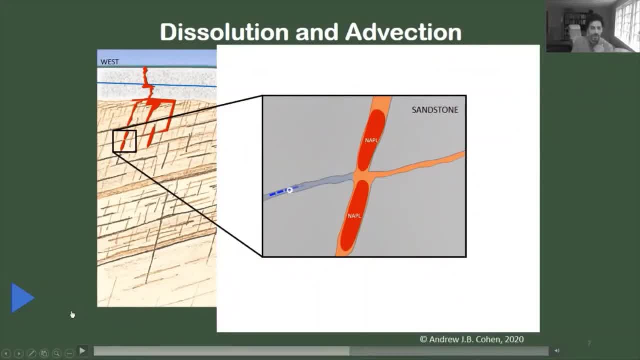 if you will right, And that's migrating in the direction of flow, And at this point the groundwater is clean, right, There's no contamination. However, it makes its way near the DNAPL, where there's now dissolved contaminant. 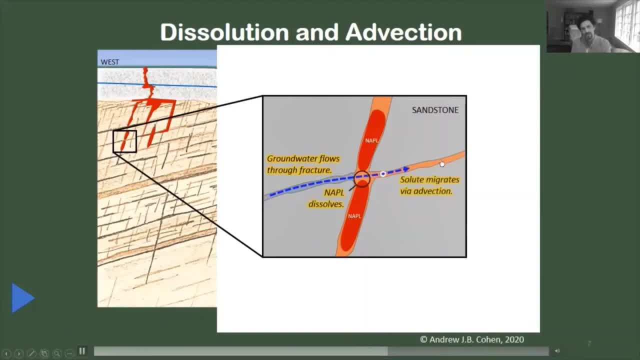 and groundwater to the right of this or downgrading, is now contaminated. Okay, so take a look at that a couple times. So again, here are our globules. it's dissolving into the groundwater. this package of water flows through it. it's not contaminated, right? So you've got. 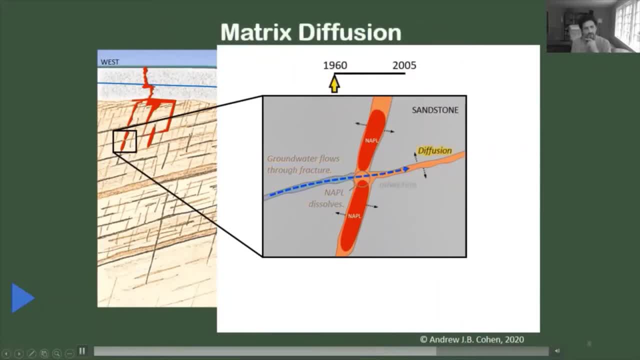 advection, you've got dissolution and now we have a case where, essentially, you have these globules of waste, liquid waste, let me call them. let me call it trichloroethylene, okay, TCE, So that's dissolving into the water, immediately around it and in these fractures. 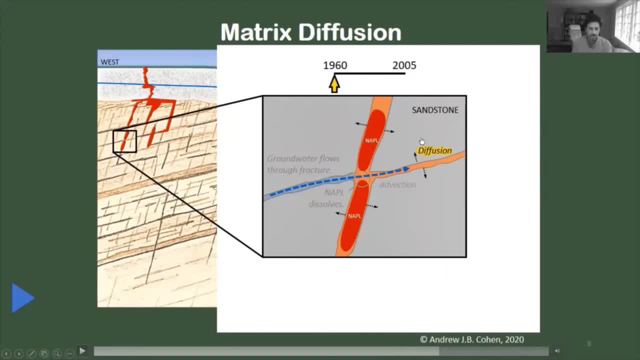 So as a result, again, the sandstone is porous, So now we have higher constant and it's filled with water. So now we have dissolved constituents here. it's then going to diffuse into this rock matrix. So what happens? Imagine we've got a spill starting in 1960,. 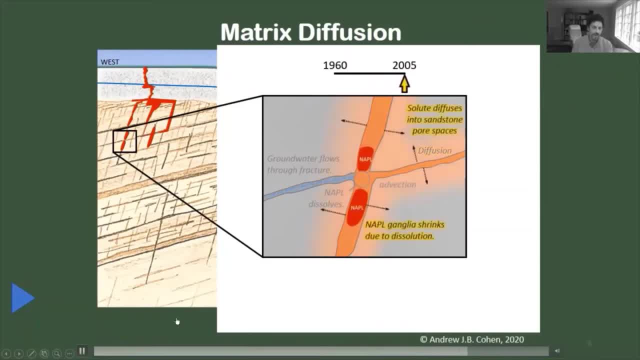 this material starts dissolving into the rock matrix and, just by way of the fact that mass is the rock matrix, these ganglia are also shrinking. okay, so this is a. this is an example of source of a contaminant and its fate and transport, or, if you will, it's transporting fate. so here we. 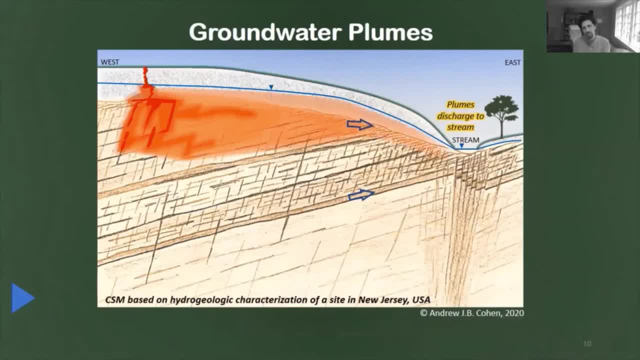 kind of summarize it up. we've got the source of dean apple. groundwater is flowing, it results in a groundwater plume. it's, it's a. it's a diffuse plume because of the diffusion and and because of the matrix diffusion which i just showed, these plumes are discharging to the stream, as you can. 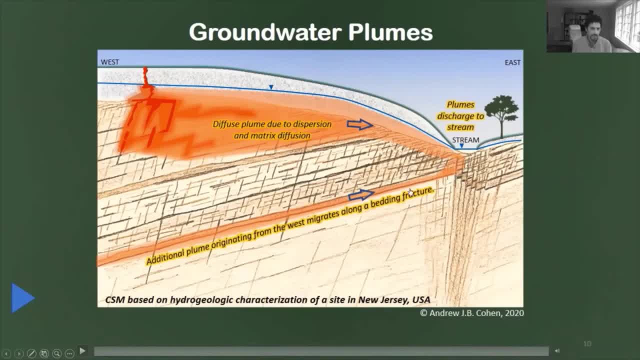 see there's a separate plume here which commingles, and this is from maybe a source farther to the west and it's just migrating along a particular bedding fraction. so there's a lot of stuff going on here and when you go at, when you, when you go to a site and you try to figure it out, you're really doing. 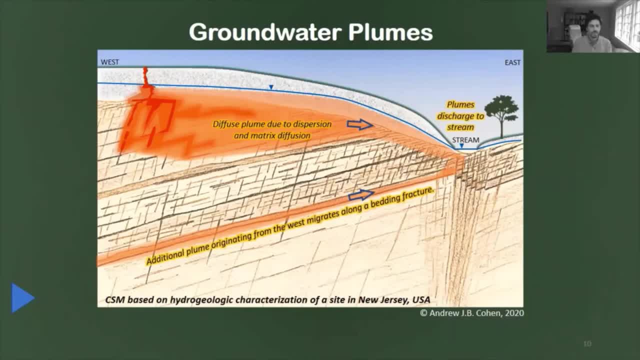 it's a very interesting combination of disciplines. you're dealing with geology, you're dealing with chemical chemistry and hydraulics and in some cases you'll do some numerical modeling. so for those of you who who might find this interesting, it is kind of an exciting field. 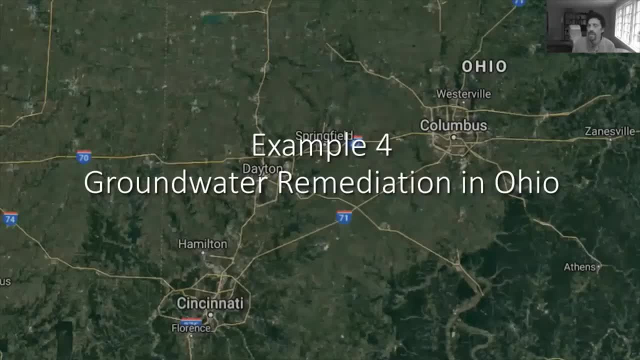 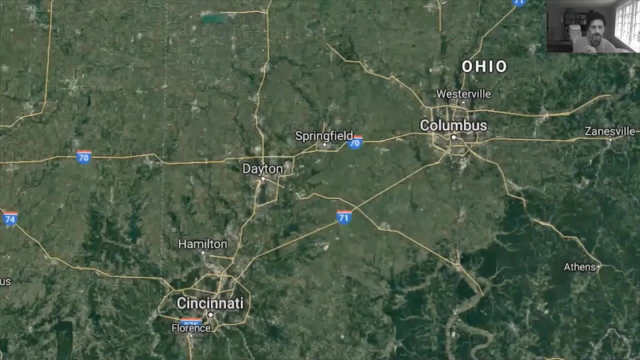 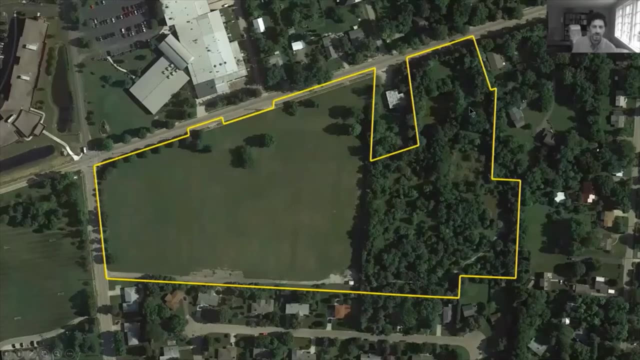 okay, all right, let's look at groundwater remediation scenario in ohio. this is close to dayton, just a few miles outside of dayton. this is a property boundary of an old facility where i believe they were manufacturing uh plastic tubing and they did use solvents and, as a result, they had groundwater contamination. 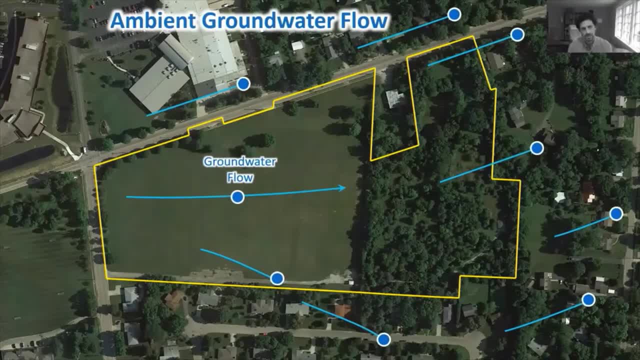 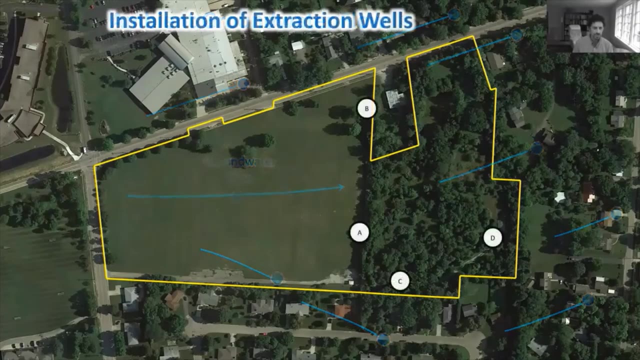 so, essentially, when you look under ambient conditions right before any wells are installed or anyone starts to pump the water, the groundwater is essentially flowing towards- towards the east in this case. because of this contamination, they decided to install a number of extraction wells- four extraction wells- and the purpose of the wells was to essentially 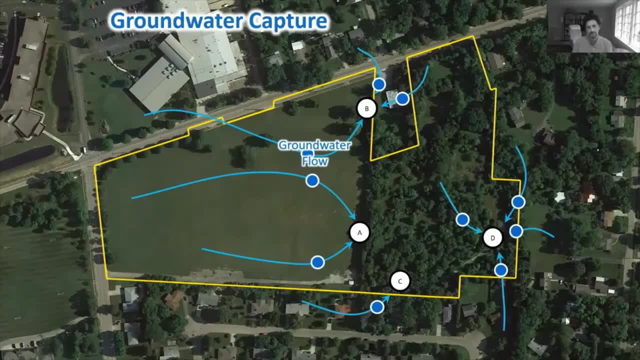 contain the groundwater, so that groundwater no longer was able to flow off-site because there was essentially groundwater contamination. they wanted to prevent further off-site migration by way of installing these, these traction wells and these flow directions i'm drawing are based on measurements of water levels throughout the site and 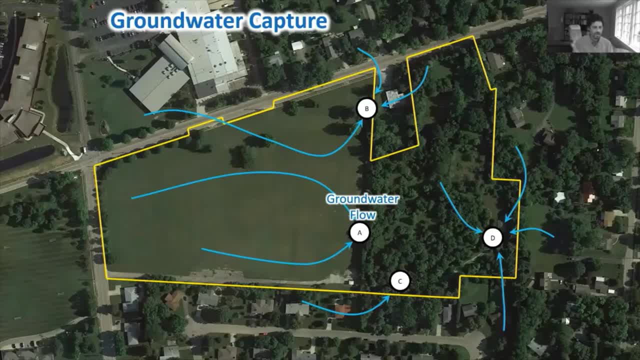 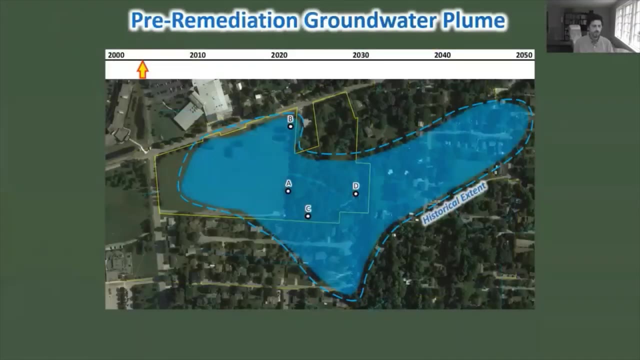 interpolated um potentiometric maps and resultant flow direction. so these flow directions are just don't come out of nowhere. this is based on an analysis of water levels collected in many wells which are not shown here. so here's the plume, the groundwater plume, as you just see here. i'm just 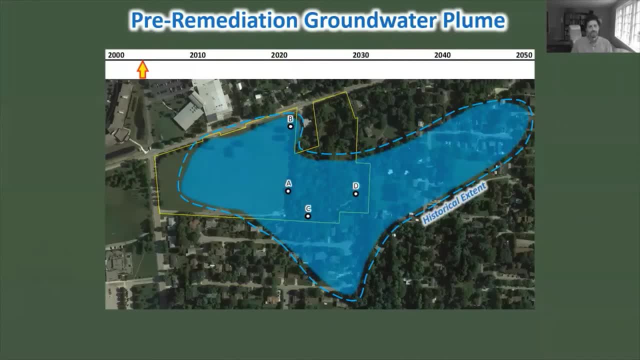 doing a single color to denote the lateral extent map view. this is the scenario in about 2004, something like that. this is prior to remediation. the plume has migrated off-site and they started to pump these wells, pull in the water and, as a result, this plume is shrinking. right, you do get. 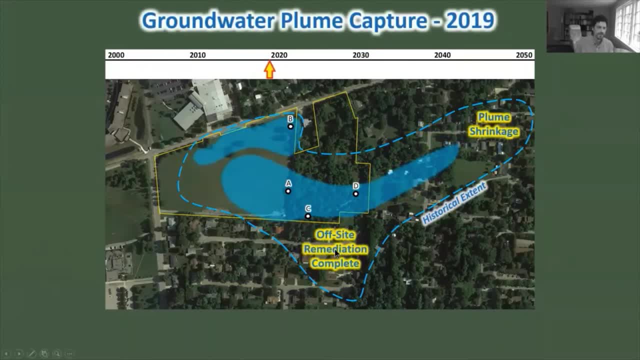 off-site remediation is complete. that's basically pulled it in and farther down gradient. it hasn't pulled it all the way in, but certainly it has been shrinking. now to: as part of the remedial plan, we did some numerical modeling and found that it would take about 20 plus years. 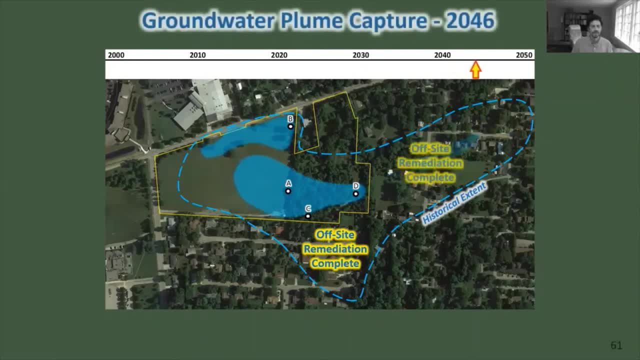 for the contamination to be fully contained on site. okay, so that's by way of some numerical modeling. okay, now we see by 2046 we'll have complete off-site remediation. in fact we just took some or some. some recent sampling was performed and it looks like the offset remediation will. 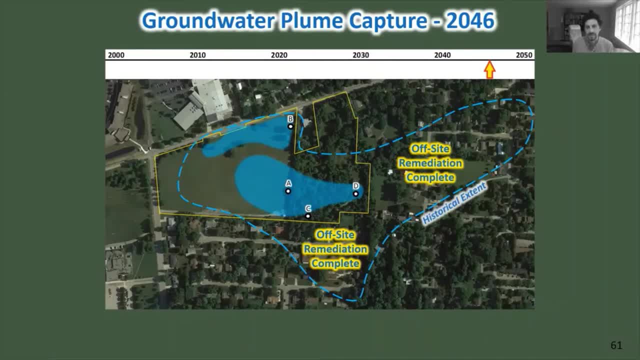 will happen much sooner than 2046. that's, the community is pretty happy about that. so you can see that one of the one of the benefits for this visualization is the community, the public, the regulators, the stakeholders. they're gonna have a very difficult time understanding what's going on without some kind of illustration. in this case it's in the form. 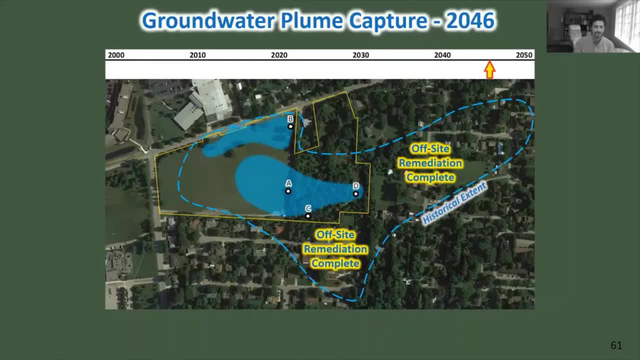 of animations based on, based on data and collection of data points that i'm not showing here, and this is really helpful for them to understand what the problem is and for them to essentially buy into whatever suggested remedial approach that you present. Okay, let's take a look at, I think, the 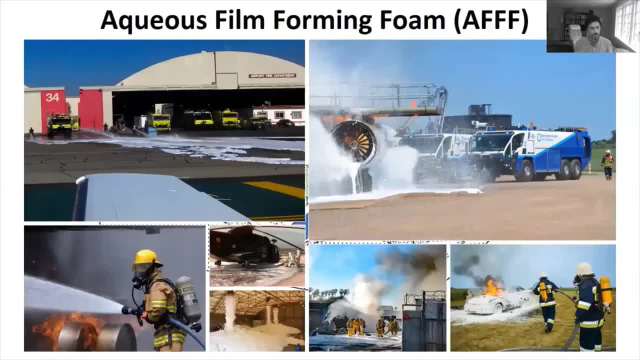 final example. this is contamination by firefighting foam, also called aqueous film forming foam or AFFF- Again hot topic. this is used, or has been used, ubiquitously at airports, military bases, and you can see that here they're just doing a nozzle test, nozzle spray test. the foam is 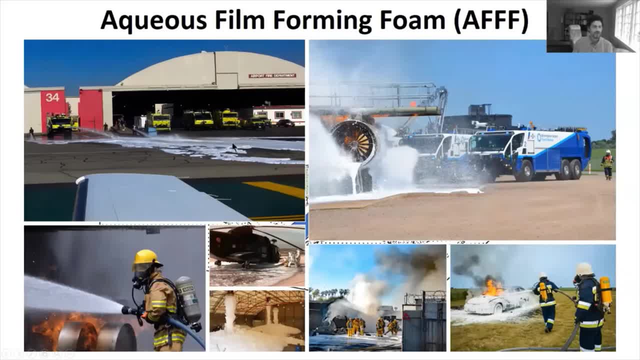 you know this is basically a foam solution. they're just bringing on the on the tarmac or taxiway. here they're doing mock fire extinguishing tests, where essentially they just have these fuselages that they line fire and pretty regularly they go out and see if. 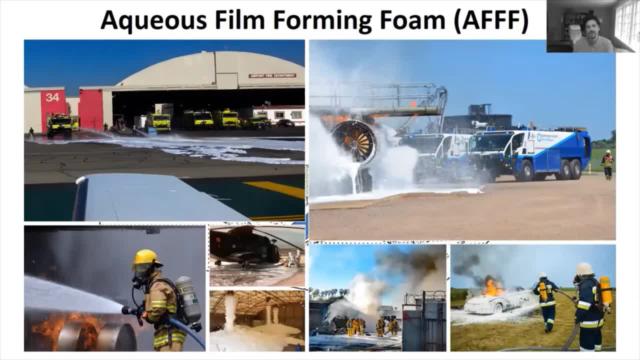 they can put this stuff out- that the unique feature of the AFFF is that it basically is the AFFF. that is the AFFF. that is the function of the AFFF. The function of the AFFF is that it It puts a layer of foam on top of a fuel-based fire. 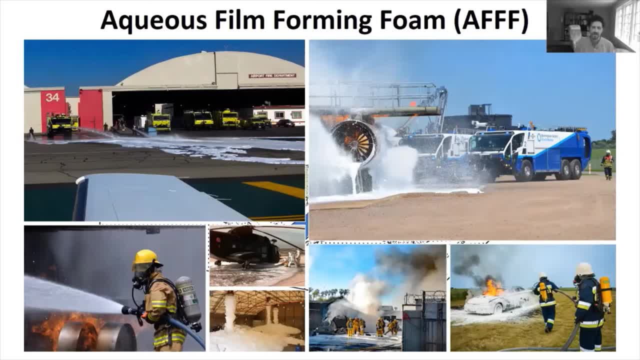 and essentially it restricts oxygen from getting to the fire. So it basically is the best kind of material to put out a fuel-based fire. In other cases they use it actually when there's an accident, but not only when there's a fire. 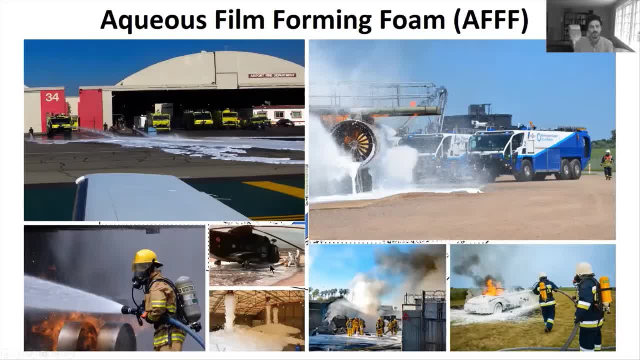 If there's just a fuel release, they'll use the AFFF okay. So you can imagine there's a lot of AFFF around airports. In hangars they've got these large dispensing systems where, if there's a fire, this stuff just comes gushing out of the top of the hangar. 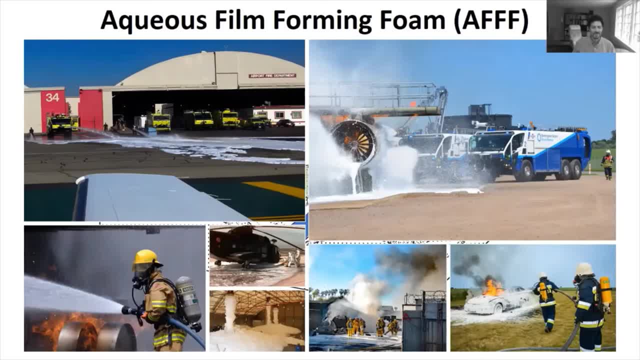 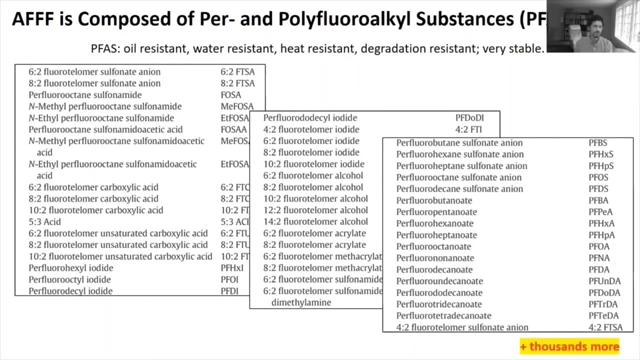 and just covers by many feet thick of AFFF. Here's some usage of actual fires. This is probably a mock scenario. So what's special about AFFF? Well, AFFF is composed of per and polyfluoralkyl substances, right? 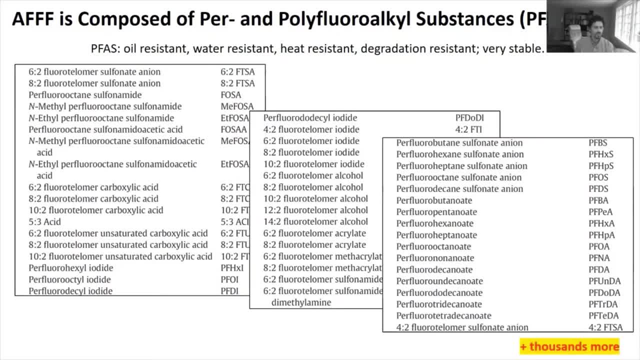 Or PFAS, And these are unique because they're oil-resistant, water-resistant, heat-resistant, degradation-resistant, They're very stable And there are thousands of them of various molecular constructs, And probably the ones that are getting greatest media coverage are PFOS and PFOA. 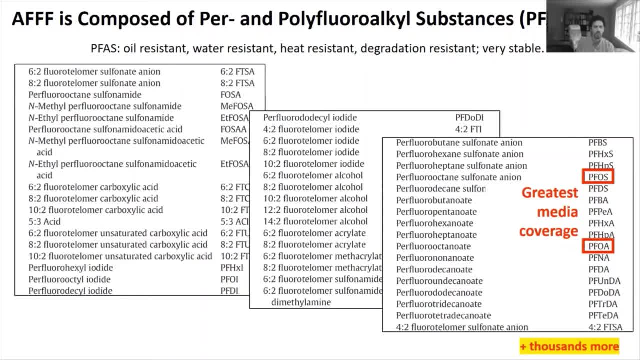 or PFOS and PFOA. okay, But you're hearing more and more of these Regulators are requiring sites or responsible parties to sample their groundwater and analyze them for 30-plus chemicals, various chemicals, And they're setting extremely low groundwater quality standards. 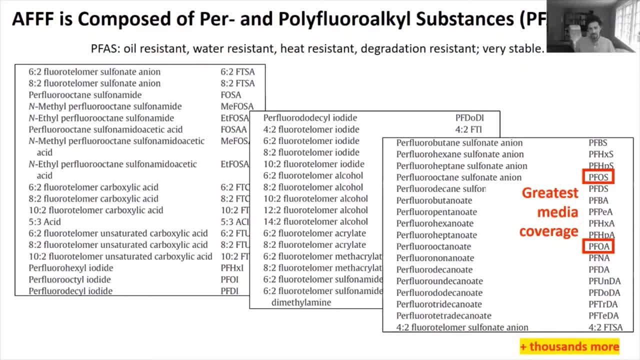 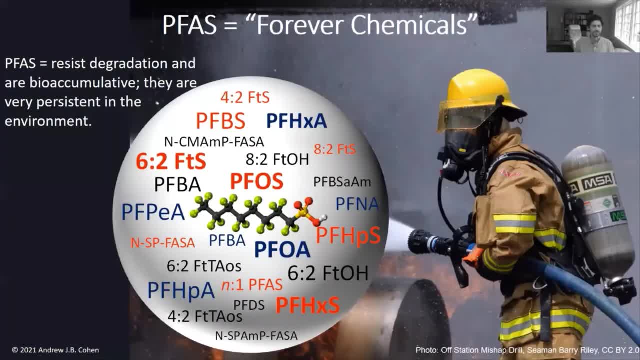 and the PFAS are referring to the PFOA and the PFAS are referring to as forever chemicals. Like I said, they're very stable, They resist degradation and they're bioaccumulative in the environment And, interestingly, in the water environment. 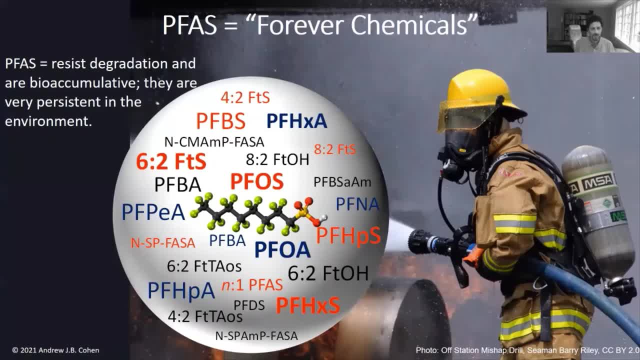 they're different than, let's say, metals like mercury which, as you may know, in fish bioaccumulate in fat tissue. For PFAS they actually bioaccumulate in muscle tissue And, again, very recalcitrant okay. 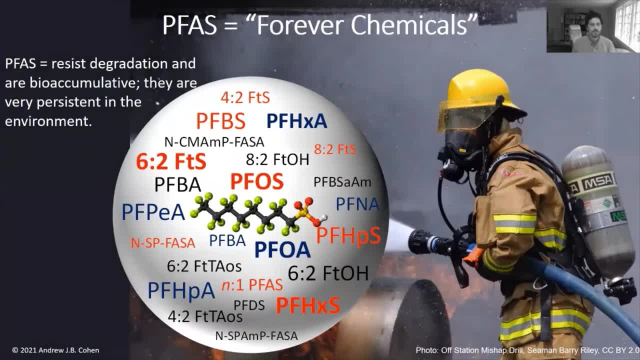 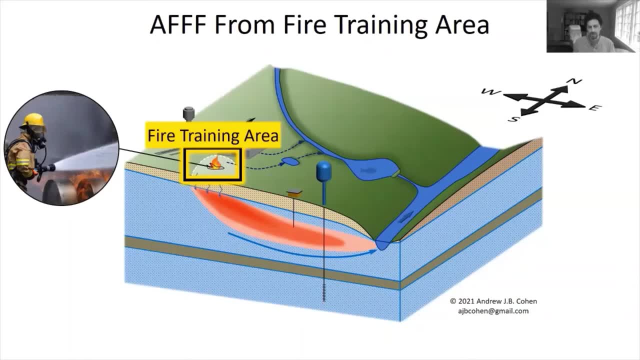 And they just build up in the food chain. So let's take a look Conceptually to get an understanding of what goes on when we're using the AFFF. So here's a similar oblique view of a groundwater system. Here's a fire training area, fuselage on fire foam around it. 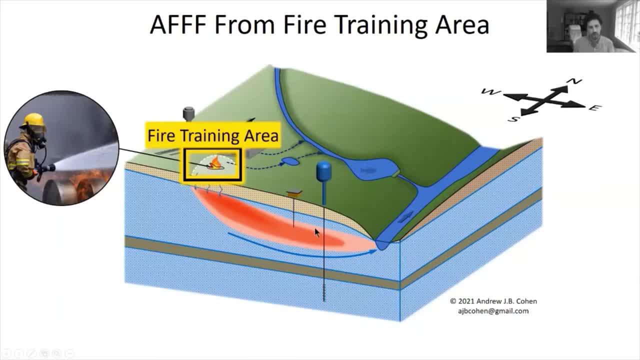 That's then infiltrating and creating a groundwater plume. And just a note here: like I noted previously, the colors are just used to denote relative concentration. In fact, the AFFF is colorless. You can't really see it at all. 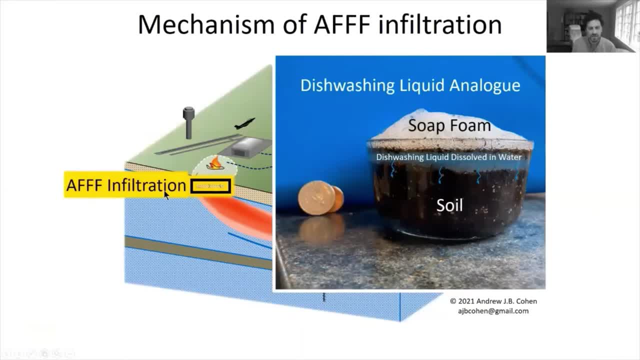 And note that this plume is discharging the surface water. Okay, let's talk about the infiltration. So we were talking about foam. This is important. I'm not talking about foam infiltrating the ground and resulting in a plume. I'm using this dishwashing liquid analog. 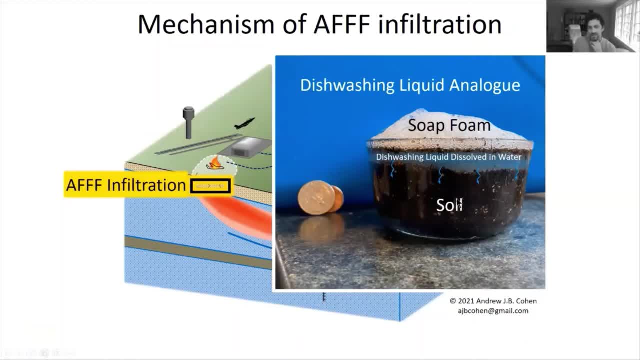 This is just something I put together in my kitchen. right, Here's a glass dish. I put some soil on here, I mixed in some dishwashing liquid And I basically agitated it right. So you've got some soap foam floating on top. 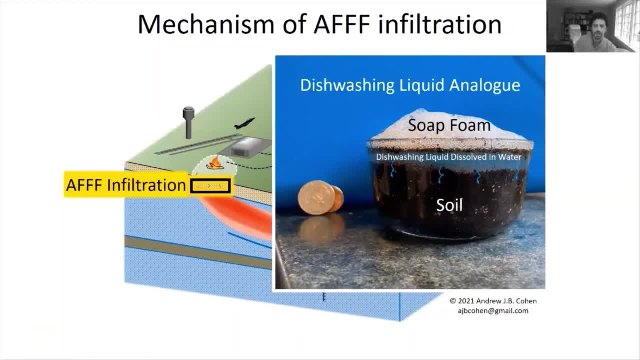 Beneath that and the soil, you've got dissolved liquid soap And it's that dissolved colorless liquid that's now infiltrating the soil and getting into the groundwater. So that's what we're talking about. We're not talking about a foam penetrating. 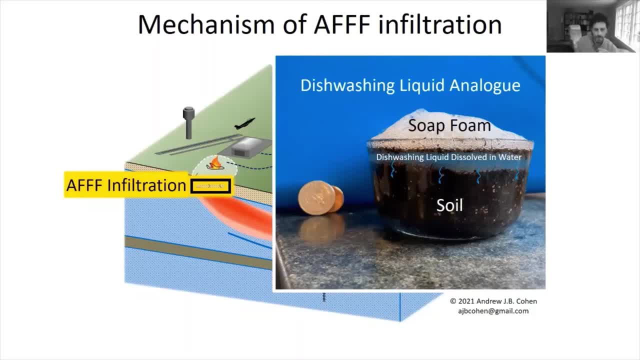 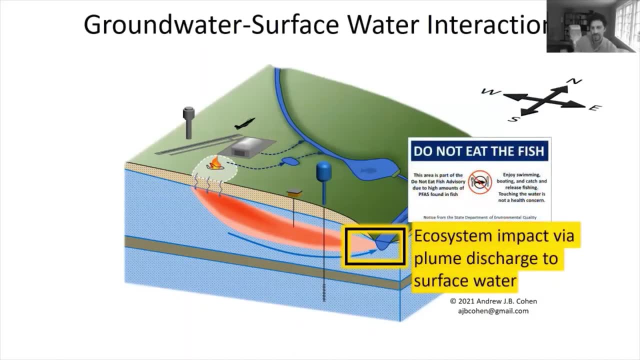 We're talking about a solute, okay, migrating in the groundwater. Okay, now this plume discharges to the surface water. It impacts that ecosystem And at sites like this, a sign just like this: one is not unfamiliar, okay. 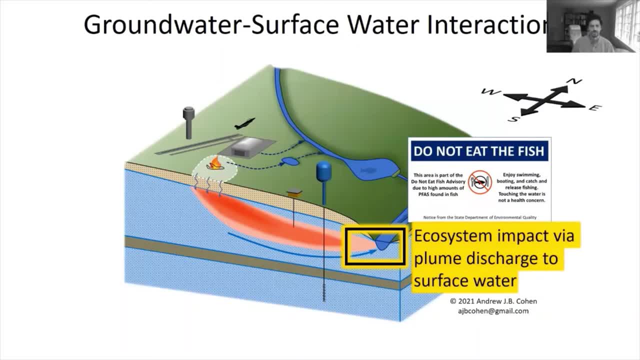 It's a common sight, especially at these military bases, right? They're telling you: don't eat the fish, So it's an issue, okay, And now it's at every military base and pretty much at every airport and also at Petroleum refineries. 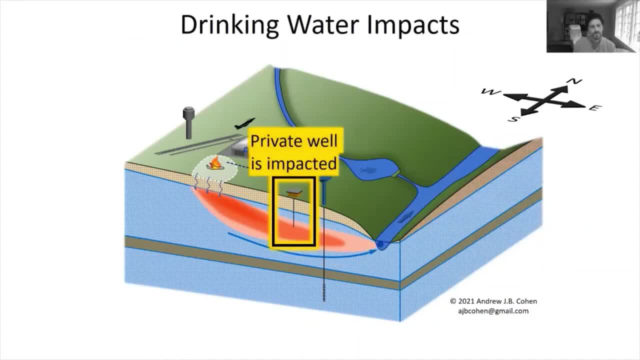 So similar to before. we've got a shallow well here. that's basically extracting water from the plume. That's impacted In this case. I talked about unconfined and unconfined aquifers. In this case, the deep municipal well is tapping into the confined aquifer. 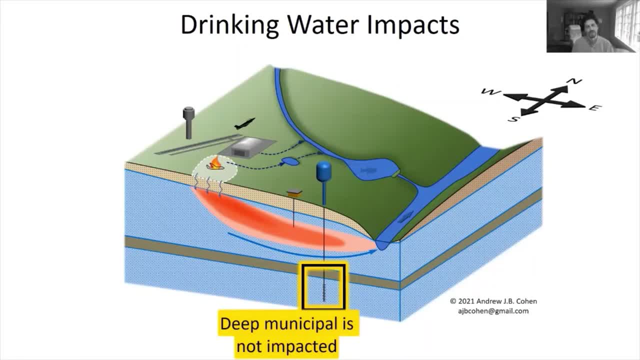 So it's not actually impacted by this PFAS. So that's important to keep in mind. Just because you might have groundwater contamination, it doesn't necessarily mean that your municipal water supply is going to be impacted. It might very well be the case, but don't just jump to that conclusion that 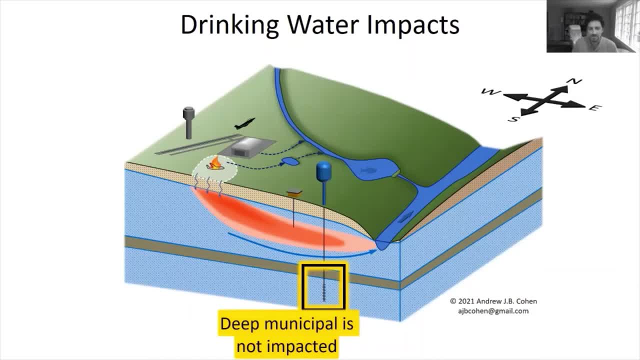 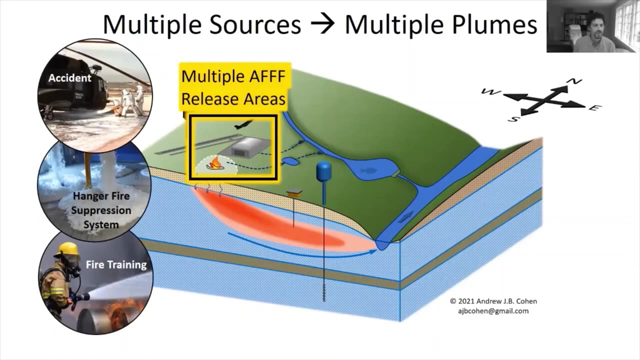 hey, groundwater contamination is going to result in impacts to our municipal water supply. Okay, I talked about just the use on the fire training area, but really there are multiple sources. right, You've got the accidents. You've got the suppression system in the hangars. 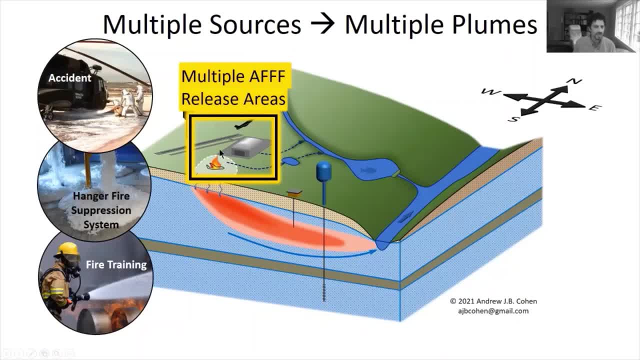 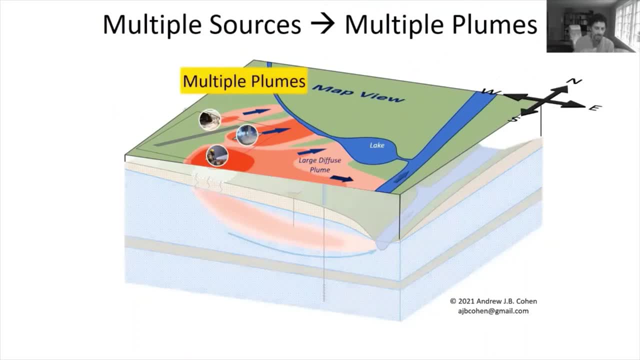 And these are in different areas: multiple releases and that's going to result in multiple plumes. Okay, so this is now showing a map view of all of the plumes. We don't have just one plume, It's many plumes. 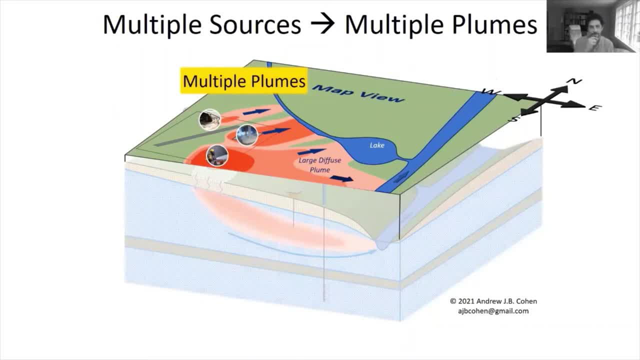 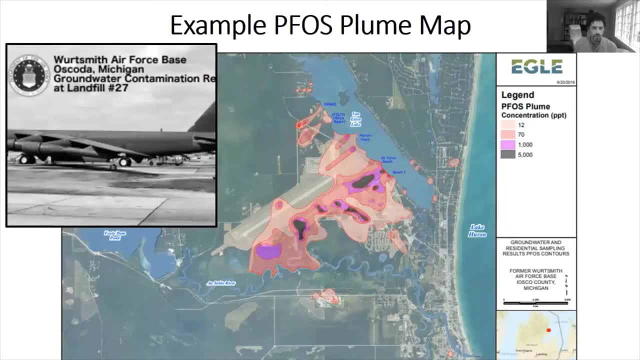 And in this case they're all discharging to some kind of surface water body. A good example is a very well-known Air Force base. It's based in Michigan And you can see here- I believe the scale is something like: 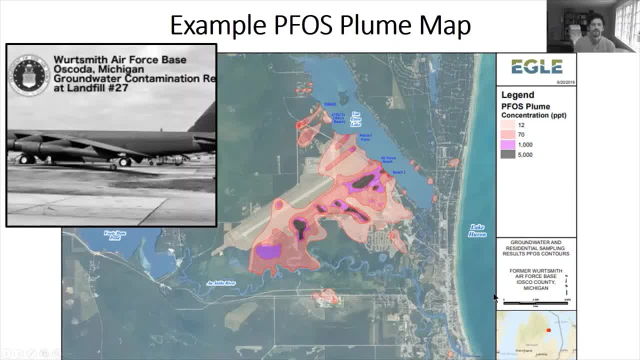 I can't quite make it out. Maybe it's 4,000 feet this whole thing. They've got multiple plumes all commingled from various sources. You can see here this one hotspot That's from a particular accident where they sprayed the AFFF. 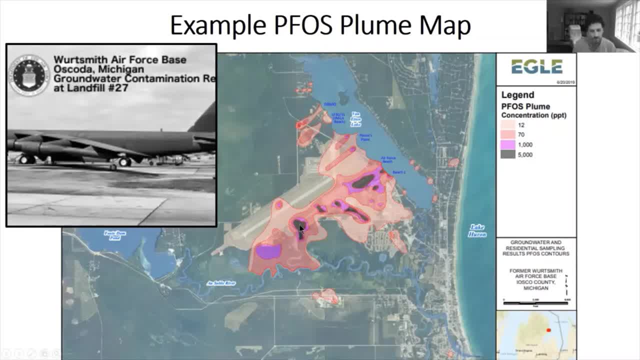 But there are many other hotspots which resulted in groundwater plumes. This plume looks like it's migrating to this surface water. These plumes are migrating and discharging into this surface water. Okay, So clearly a big issue here, And these concentrations are many orders of magnitude higher. 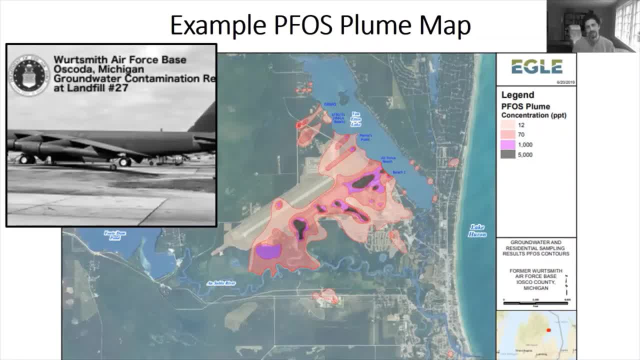 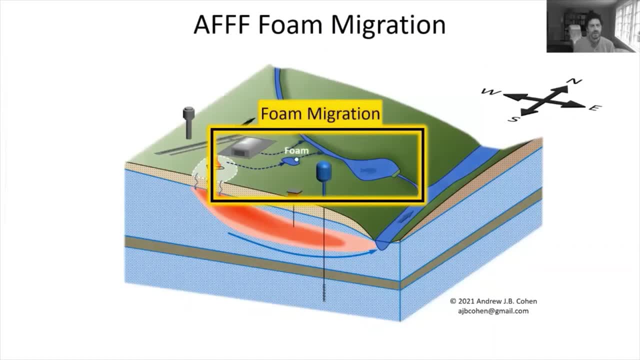 than what are considered safe concentrations, So clearly an issue in some places. So let's just talk a little bit about the foam migration. I showed you the foam in a little kitchen experiment. That stuff is floating on surface water into reservoirs. 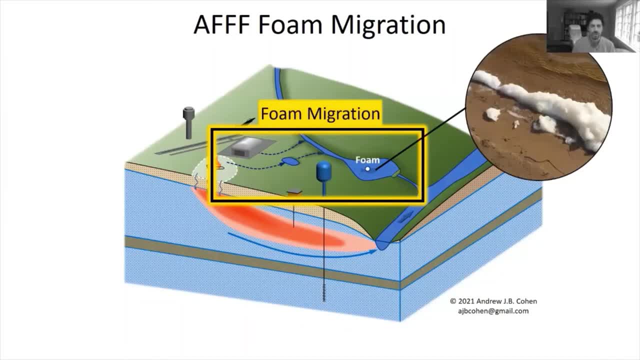 And you wind up seeing the foam just washing up on the shoreline. I do want to note that, So that foam is common in surface water bodies. It's a result of basically the biodegradation- just natural organic material, And it does result in some foam. 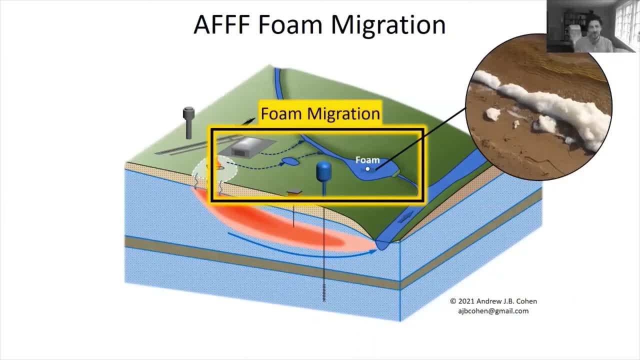 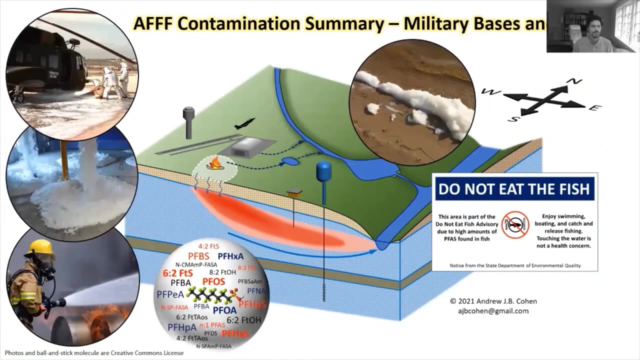 So just so you know, if you see some foam in a surface water body, don't assume it's AFFF contamination. It could very well just be naturally occurring foam. So AFFF summary: we're talking about military bases and air porous. 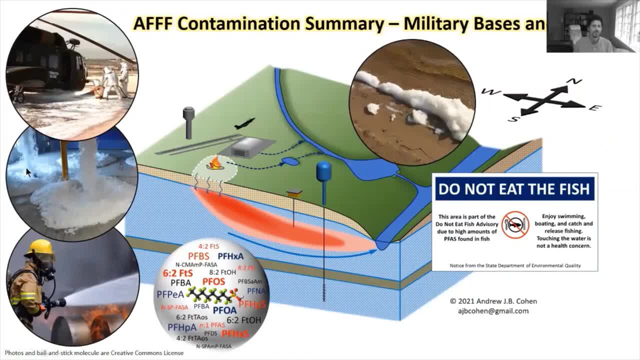 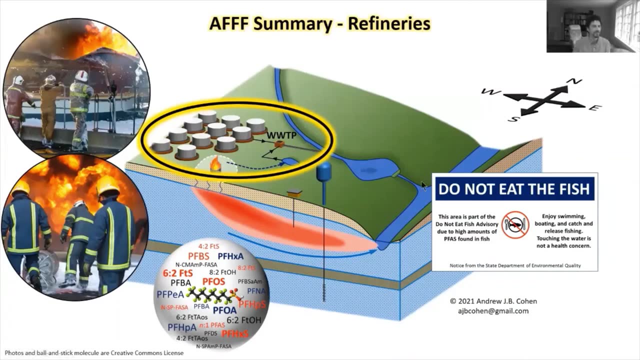 I'm showing the chemicals that we're talking about, the various sources We've got the plume: discharging to surface water, occurrence of foam and the ecological impacts. Now something similar occurs at refineries, because they're also using AFFF to put out refinery fires. 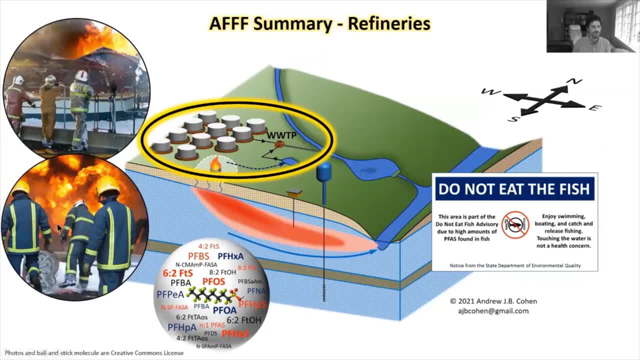 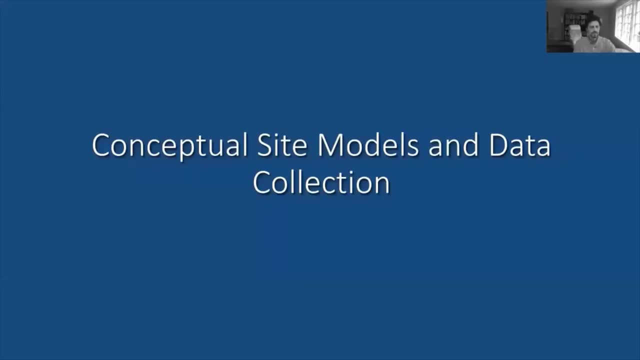 I mean, look at this fire. This was absolutely massive fire. They're using thousands and thousands of gallons of AFFF. I think you can see some right over here. So similarly, you do have ecological impacts. Let me see, I think I have about five more minutes. 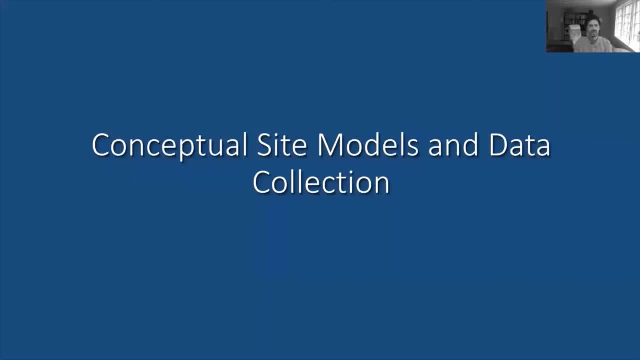 Let me just take you through. Is that correct? I have five more minutes. OK, I'm going to assume that I do. Yes, sorry, I came closer so you can hear me. Yeah, Maybe like two or three, so we have some time for questions. 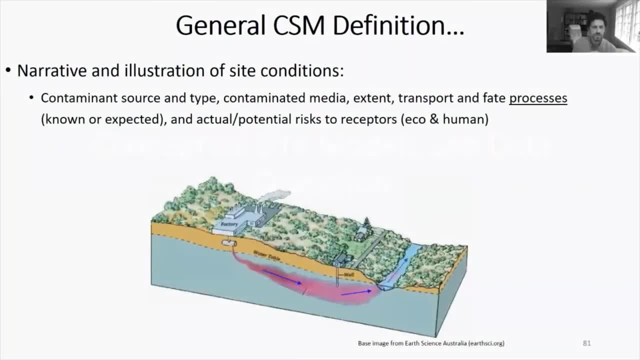 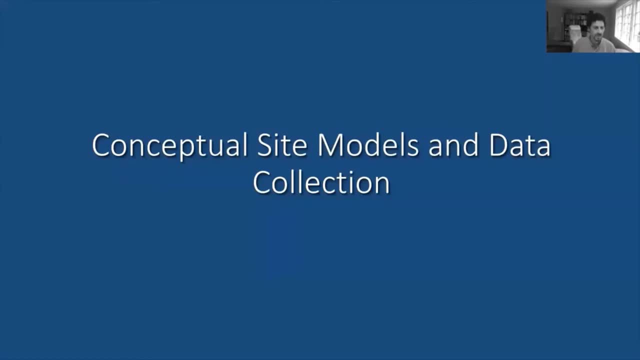 OK, Let's do two or three, OK. So what I've just showed you, the examples I've shown you, I've shown you the different types of AFFF, What I've just shown you are essentially what are called conceptual site models. 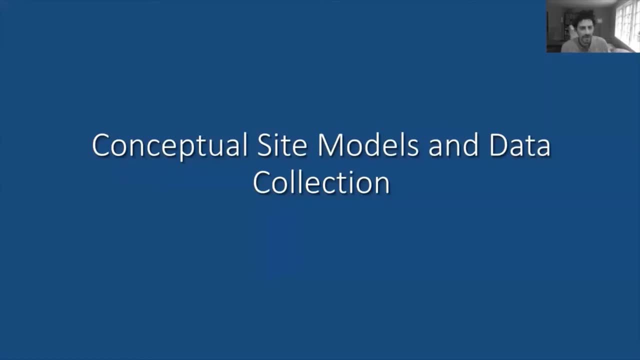 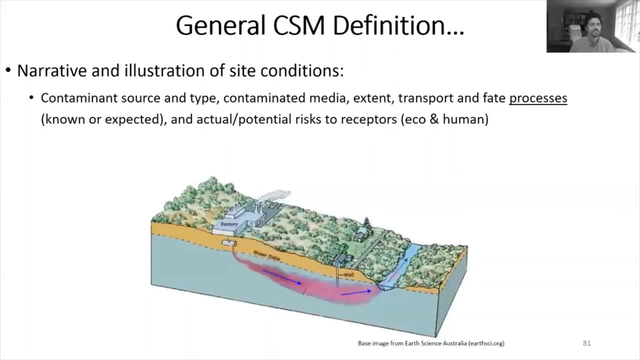 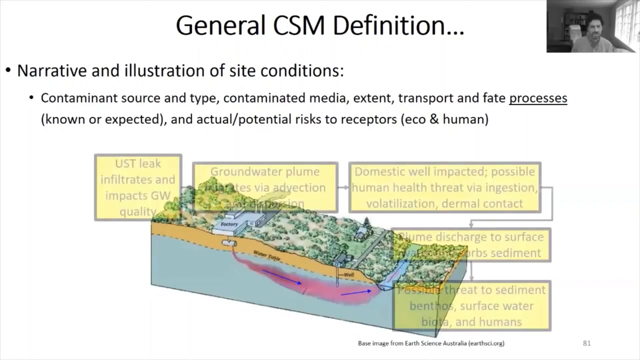 They're not actually showing the data. They're showing the result of the data interpretation and providing a conceptualization of what's going on. OK, And so, generally, a conceptual site model. it's a narrative, an illustration of site conditions. It's essentially what I just did. 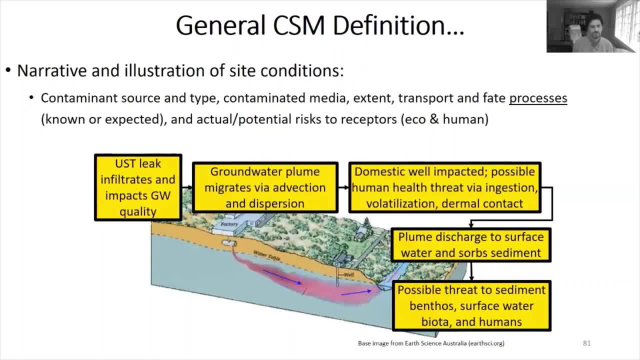 It's kind of some illustration of what's happening and a description of where the sources are, what the migration characterizes, And so I'm going to show you what the sources are, what's impacted, what are the fate and transport mechanisms, and are there actual impacts? 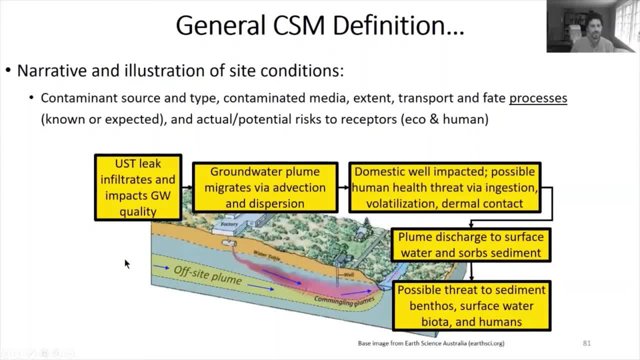 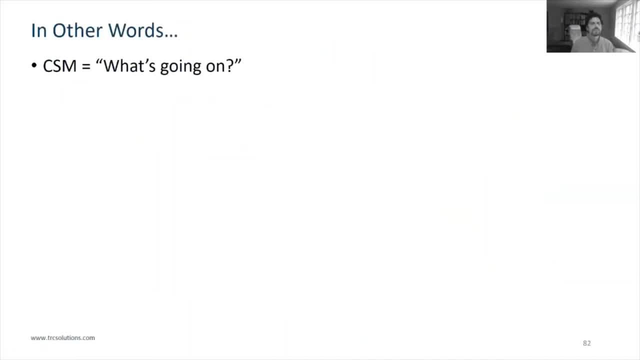 In this case I'm showing a leak from an underground storage tank, but also some plume originating from some other location. OK, So conceptual site model: essentially is what's going on, but more precisely, what do we think is going on? 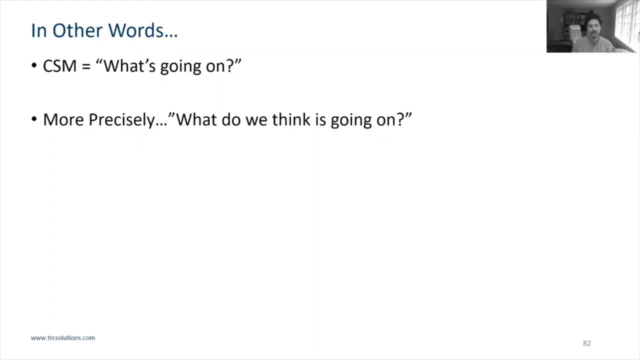 Because really what happens is we collect data, We look at the conceptual site model, we identify data gaps and then we might go ahead and collect more data, But the conceptual site model is the basis for everything you do right. It's which media needs to be addressed.